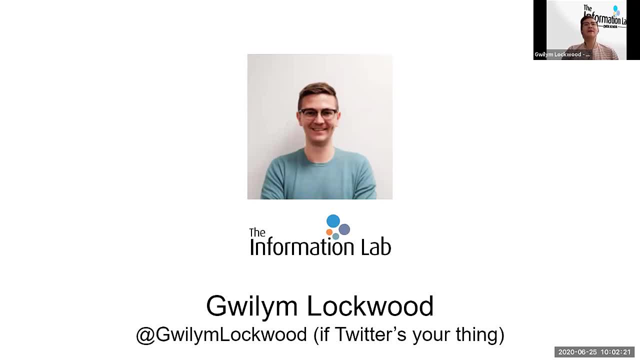 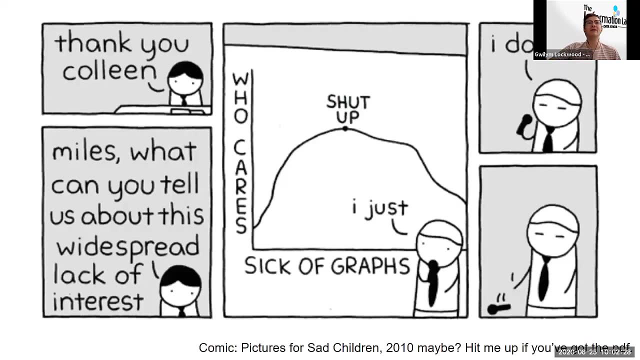 And yeah, so if I turn numbers into pictures to help people understand things, that means that I make a lot of graphs. But sometimes it goes a bit wrong and I get a reaction a bit like this: This is a. this is from a comic called Pictures for Sad Children, which I used to read 10 years ago. And yeah, the creator took everything offline, So it's hard to track it down. I'd love to be able to cite it properly. 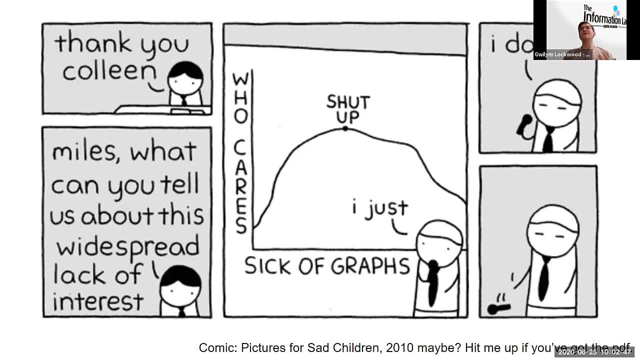 But yeah, this is just one I had saved from years ago. Anyway, this is this is the kind of reaction I get quite a lot with, more often than I'd like to admit, when I'm doing, when I'm doing building our dashboards and charts and graphs and so on. And this reaction happens because there's there's a fine line between complicated maths and stats work and simple graphics that help people understand things, And it's really easy to not tread that fine line properly. 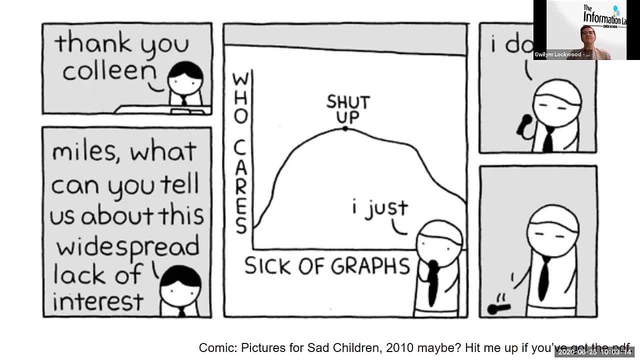 So when you oversimplify, you lose people because they can't see how you've got there. All they see is a relatively simple graph and everything about the process to get to that point is hidden. But on the other hand, if you overcomplicate things, well, you also lose people then because you've gone into way too much detail and people just want the main findings. people want to understand how they got there. but the 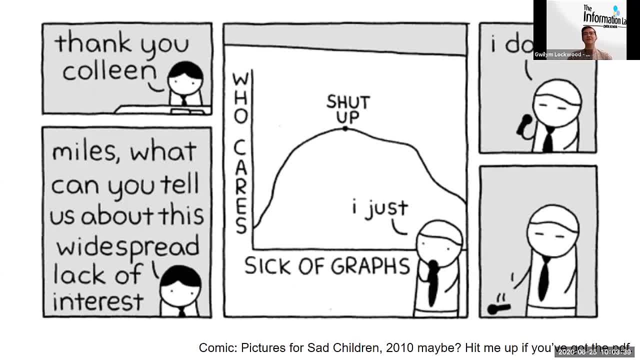 the whole process is just overwhelming and there's too much information that they just don't care about. So I kind of think of a graph as being a bit like a sausage, in that no one really wants to see exactly how a sausage is made- not exactly, but at the same time you also don't want to like a big cylinder of. 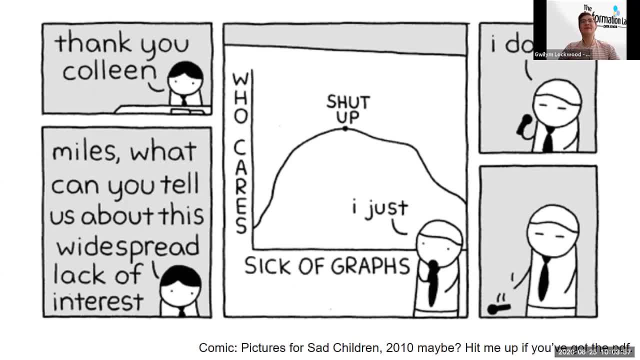 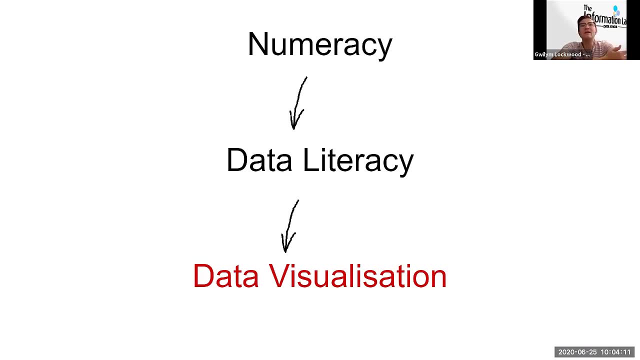 mystery meat, either of completely unknown provenance. You don't want to trust that kind of sausage either, And this session is about finding that balance between how much maths and stats to talk about in terms of what's gone into your graphs. So, working in data visualization, I often see reactions like: oh, it would be lovely to have some good data visualization going on, but we really need to sort out our numeracy or our data literacy first. This is a reaction I get from clients quite a lot. 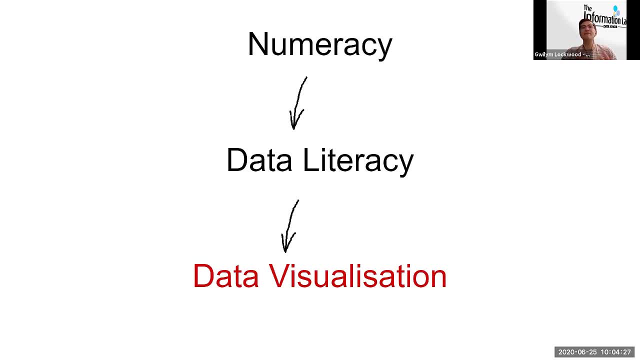 And now the perception is that you know data literacy is necessary before you can do effective visualization and you know, maybe good numeracy is needed before you can do get to the data literacy point. So you should probably focus on the numeracy first. 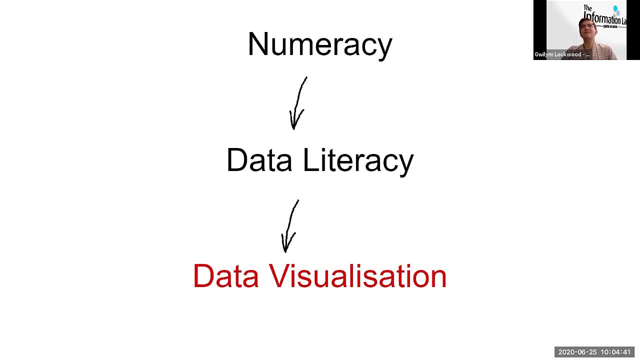 I'm sympathetic to this and I see the logic behind it, But to me it also sounds. it also just sounds a bit like: yeah, we just don't trust our people, Like even if they're not actually doing the data visualization, even if people are just consuming the data visualization to try and make decisions. 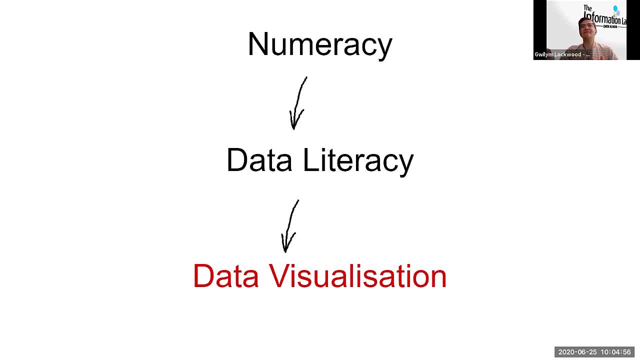 we're just not going to try and do something complicated or something a bit different or something something kind of out of our comfort zone. because of that- And to get on my soapbox for a moment- I just don't think that anybody is actually fundamentally bad at maths. 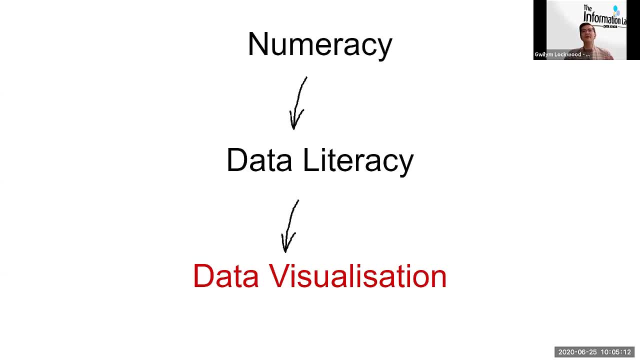 Like, maths isn't inherently hard in and of itself, but it's just that the way that maths is presented often makes it appear hard. The concepts behind maths and stats are generally pretty clear once you put it into words or once you put it into pictures. 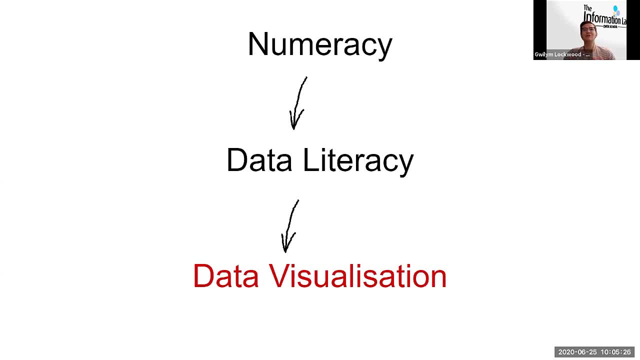 So why would you require numeracy training for people to be able to consume pictures, when you can use pictures to help people improve their numeracy? So this is why I kind of see it the other way around. I think that you can use data visualization as a starting point for data literacy and numeracy development. 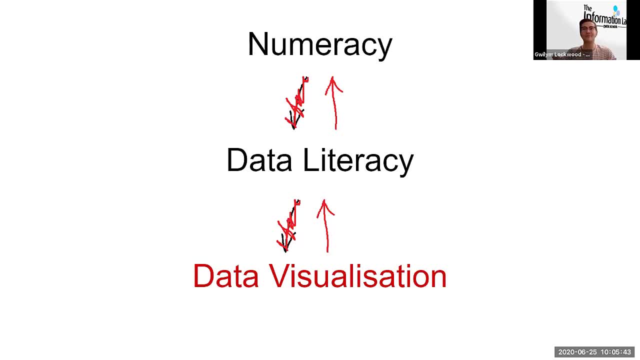 And you know, this is obviously assuming that people in your organization care about that work, because in my experience the vast majority of people do, which is great. So what better than using data visualization in your organization to help bootstrap Data literacy and numeracy? there's going to be a lot of variation in numeracy levels as well. 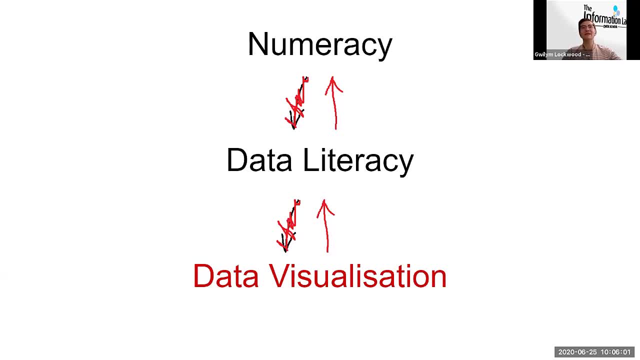 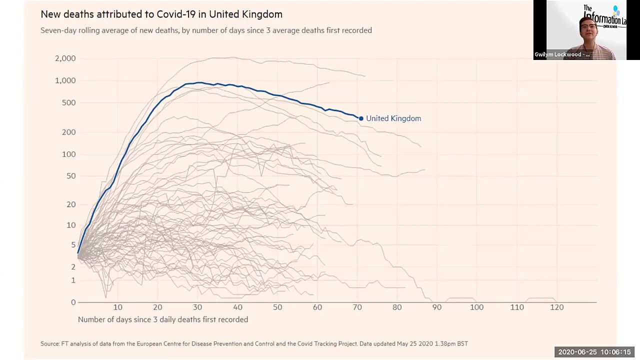 So you can then use data literacy to target numeracy and run more targeted sessions, And it's like the data visualization will lead to the data literacy and numeracy if you play it right. So we've seen this exact course play out during the COVID-19 crisis, so before February this year. it was always a nightmare to explain things like rolling averages. 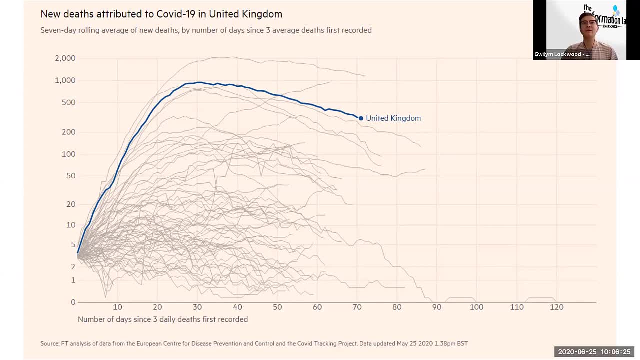 or log scales or controlling for population. You know you'd always get reactions like: well, how is this line not the actual value for a rolling average? What do you mean when it says a seven day rolling average and the line is at a thousand? 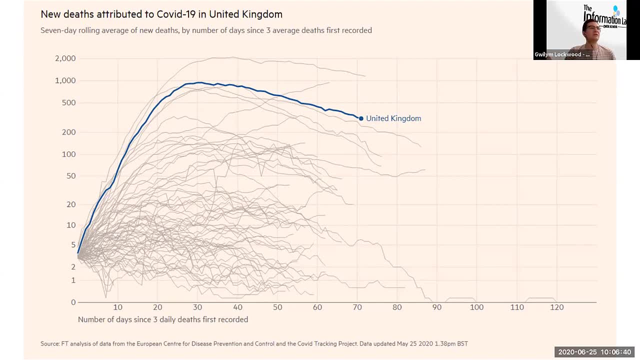 What do you mean? that? that that value isn't a thousand? I don't. I don't get it. It should be the value. Or why is the axis going up weirdly spaced? That just distorts everything. I don't understand. I don't get what's going on here. 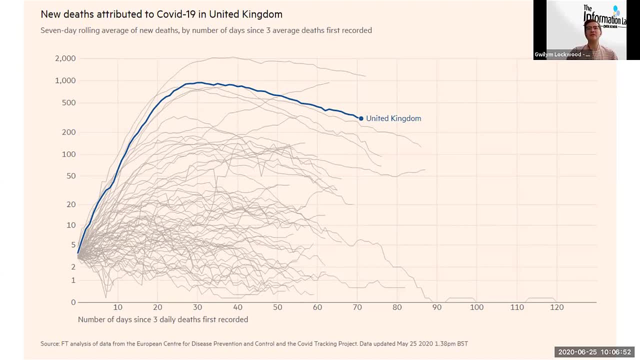 Or you're talking about, Are we talking? Are we just talking about rates or are we just talking about sheer numbers? I This is. this is something that a lot of analysts and data scientists found difficult to explain to a lot of people before this crisis. but John Byrne, Murdoch's charts for the, for the FT, among others, they've bootstrapped data literacy and numeracy from data visualization because, you know, this is a subject that everyone really cares about and is desperate to know information about. 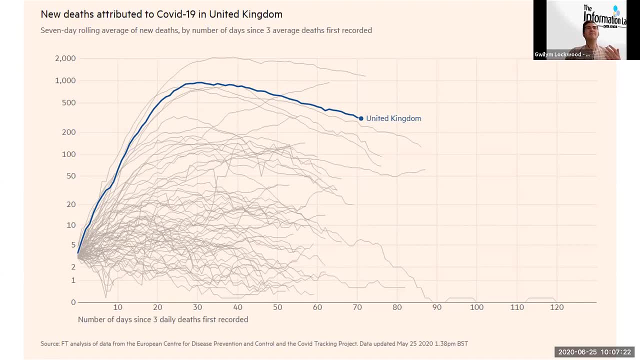 So it didn't happen the other way around. People didn't have to, People didn't see these graphs and think: well, that's far too complicated, I need to go away, attend some kind of numeracy course, attend some kind of data literacy course, and then come back to it once I reach the right baseline. 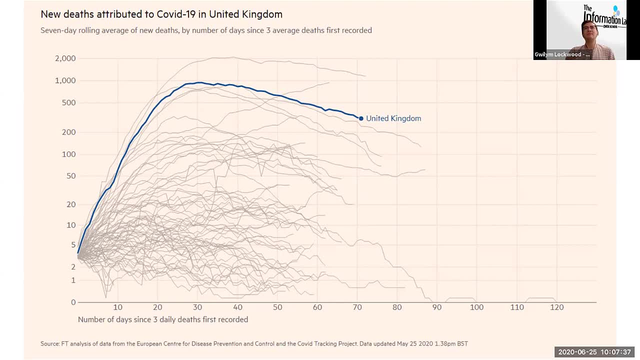 People see these charts and because it matters to them, this helps bootstrap their own data literacy and numeracy And people now get what log scales and rolling averages are, which is great, I mean. I wish it could have happened in a much more and much less scary situation. 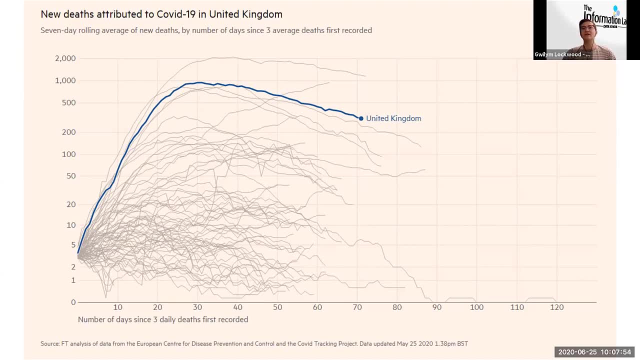 But Uh, Thousands of analysts and data scientists jobs and data visualization, visualization professionals jobs have now become so much easier. The broader point, though, is that you can do this in your own organization, and preferably with more positive data, And this is two points I'm going to keep coming back to. 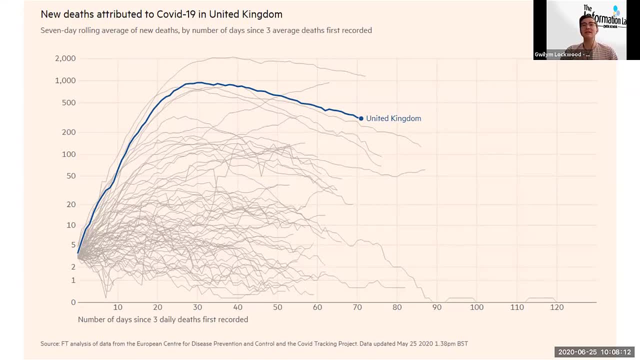 One is that people will become more data literate through exposure to data visualization that they care about, And two, you can help people become more data literate or numerous proactively With some extra explainers and sessions around your data visualizations. So let's take a simple example of how you can use data visualization in your organization to develop data literacy and numeracy. 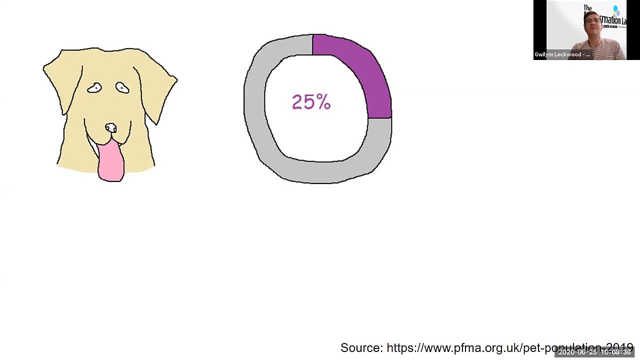 So here is my highly sophisticated dashboard of pet ownership. My donut chart here shows quite clearly that a quarter of British households have a dog. But wait, somebody else in my organization has used the same dashboard and they've sent A screenshot round via email to everybody else in the group that says that 62 and a half percent of Brits have a dog. 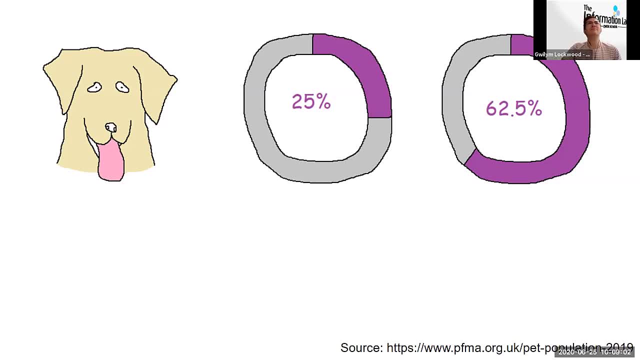 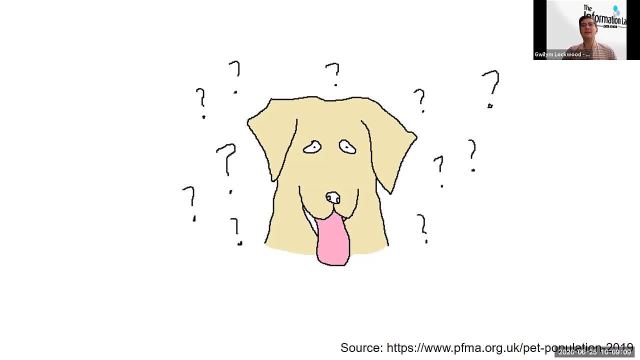 So wait, which is it? How are the numbers, not just the numbers? What's the right numbers here? It's really confusing. I don't know how many people actually have a dog. I don't know why these figures don't match. 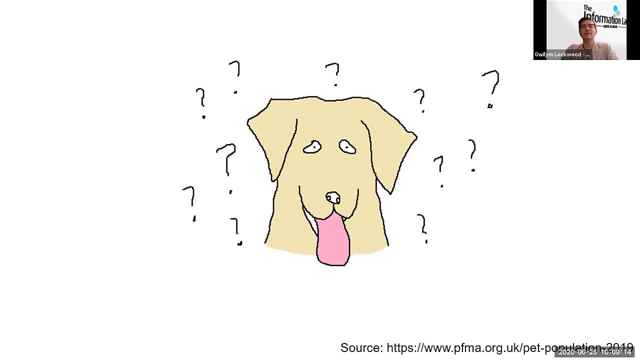 And this sort of inconsistency can be really frustrating for a lot of people. And why are the numbers, not just the numbers? And that's the problem with percentages, right, Like they change completely. Right, They change completely Depending on your level of analysis. 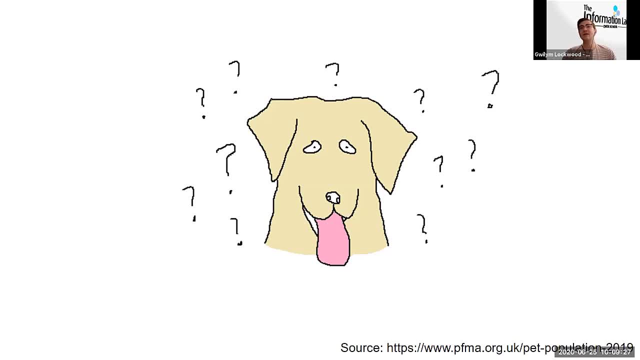 And that could be really frustrating if it's not clear what the level of analysis is. It's not a simple number. It's a number that is the numbers out of another number. that is the numbers, But depending which numbers you choose, the percentages are completely subject to change. 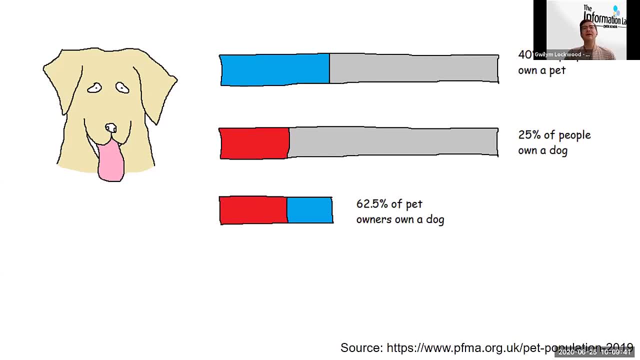 And the trick is that this pet's dashboard. it lets you filter to your population of interest. This is something I see all the time at clients. People have got a dashboard with a filter on it and they take a screenshot of it without the contextual. 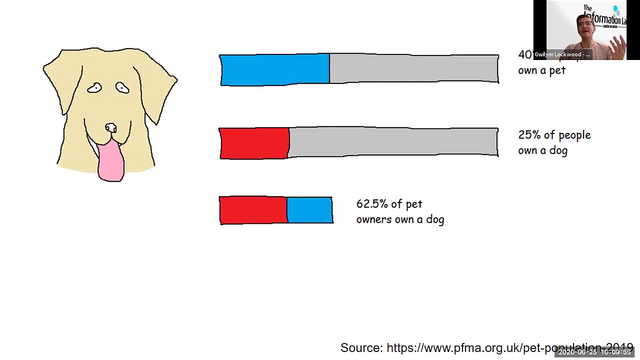 So you've got lots of just JPEGs or PNGs flying about email or Slack or whatever, with conflicting information, because people don't have the context. So yeah, it lets you filter to the population of interest. So do you want to know how many people in the UK overall have a dog, which is about 25 percent. 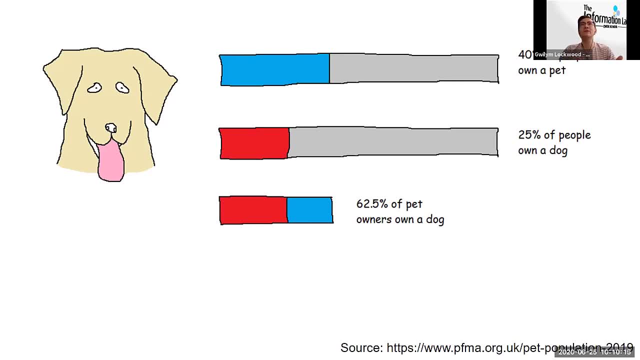 Or do you just want to focus on the 40 percent of people who have a pet of any sort, And then you can say that, of people who own pets, 62.5 percent of those people own a dog. So the underlying numbers haven't changed. 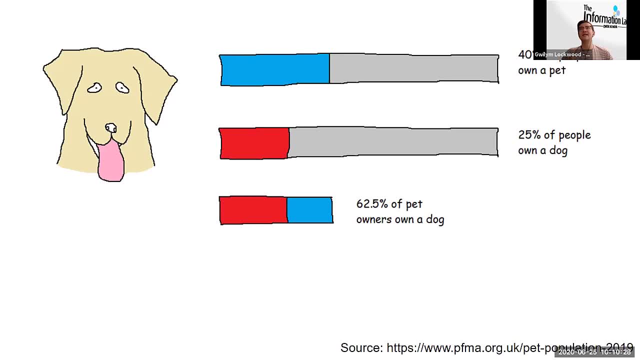 We're still talking about the same population in the UK. We're talking about the same number of people who have pets. We're talking about the same number of people who have dogs, But it's the interpretation of these numbers that's changed. It's the interpretation of the percentage that's changed. 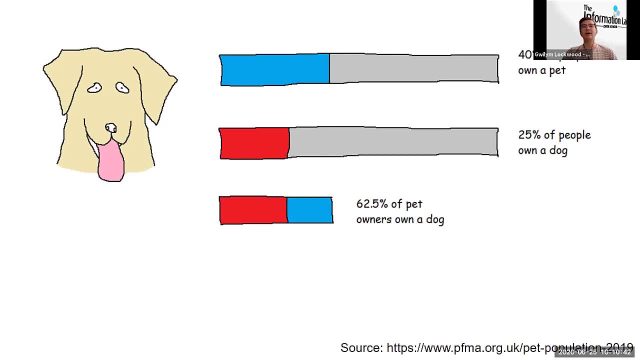 And it can be difficult at first for people to follow which context you're looking at, But when people are uncomfortable with percentages, this could be a really useful springboard to bring in some data literacy and numeracy concepts. And yeah, there's the two things I'm going 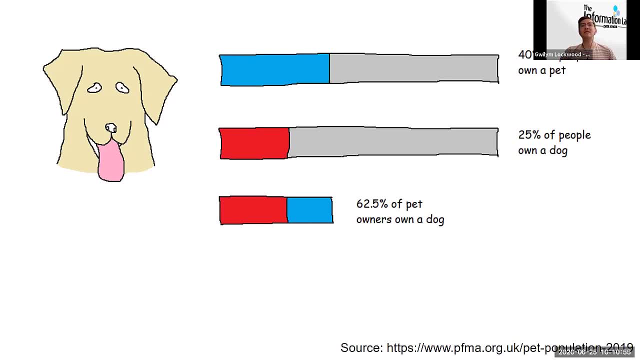 Come back to here. The first is that a lot of people will become more data literate through exposure to data visualization. So do you see how? this breakdown of totals in this bar chart? this makes it much more clear how the number of dog owners is still the same number in red. 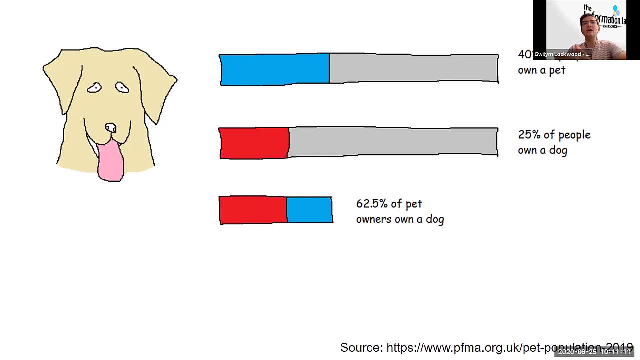 but that the percentage changes depending on whether it's out of the whole UK in gray or just British pet owners in blue. So it's much clearer to see what's going on than in the donut charts And this kind of data visualization tweak can make. 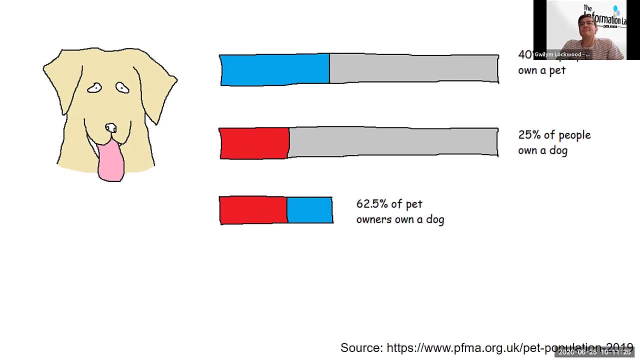 The math concepts so much more intuitive. And again, people aren't inherently bad at maths. not when you can get people to see things visually or conceptually, But also you don't. you don't just have to leave it to data literacy through exposure. 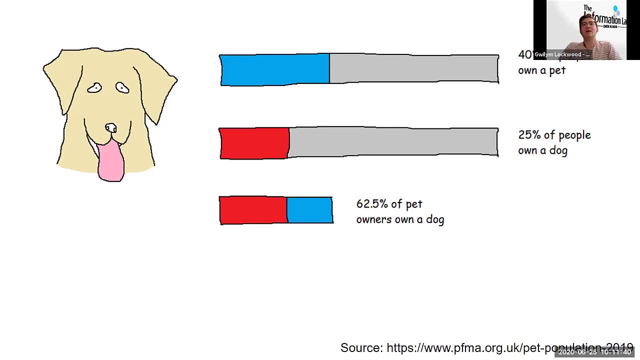 You can be proactive too. You can ask people how they're finding the dashboards. You can give them some resources for for interpreting them. You can run some hands on sessions with different groups. There's no point running generic data literacy. Excuse me, 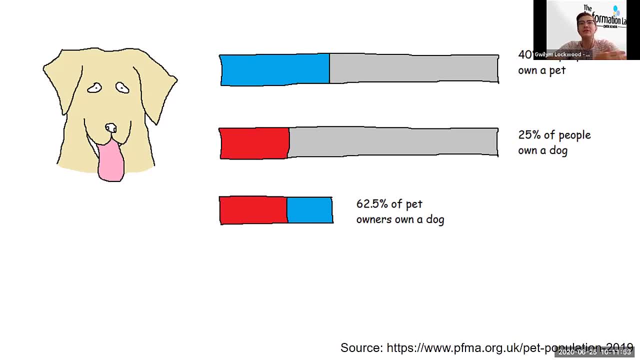 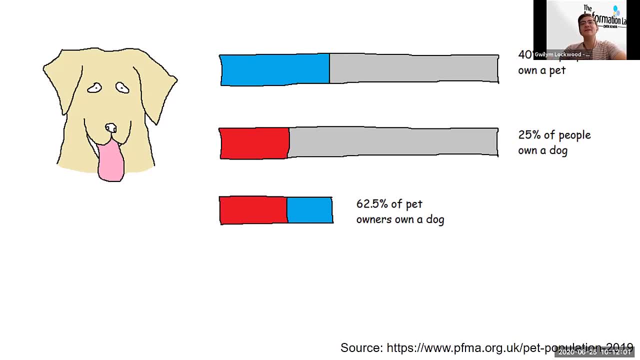 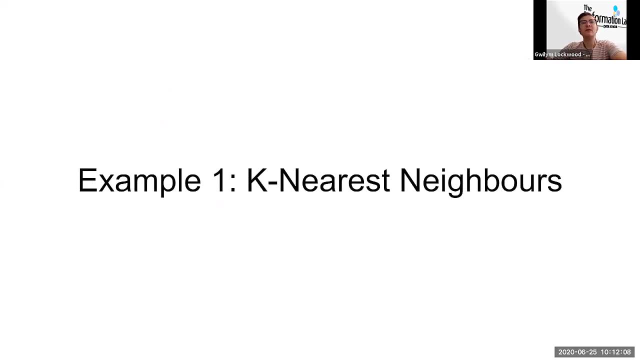 And half your people will also find it way too basic, But you can use database to get a sense of where everybody is and then run training in a more targeted way to the different groups that you're working with. So let's say I'm going to talk about some examples from from industry, where, where things are much, much more complicated than some dog ownership stats, 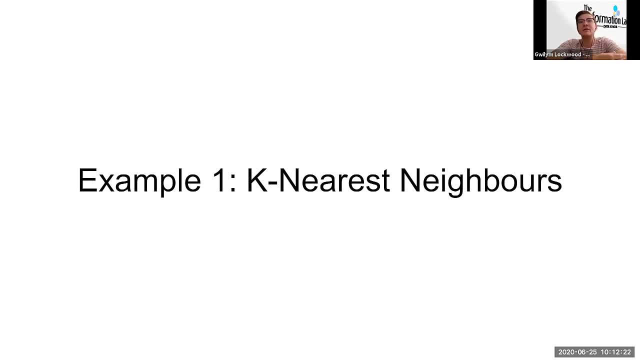 So this is based on real work I've done in the manufacturing industry. So this is based on real work I've done in the manufacturing sector. But all the data for this session has been totally, totally made up. Let's start with a K: nearest neighbors. 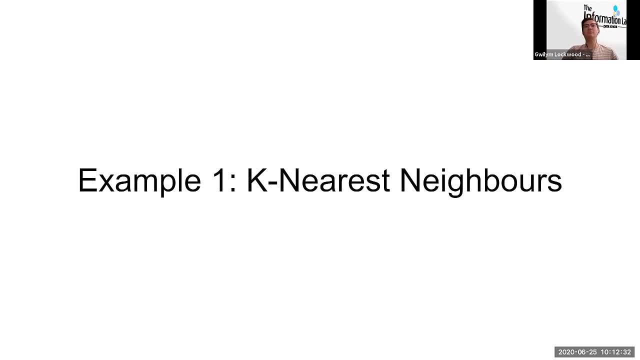 Some of you may already use K nearest neighbors analysis in your own work, But if you're unfamiliar with it, no worries, I'll just explain it quickly. It's a type of unsupervised learning technique that uses a search algorithm to look for nearest neighbors in terms of Euclidean distance across multiple dimensional space to classify things. 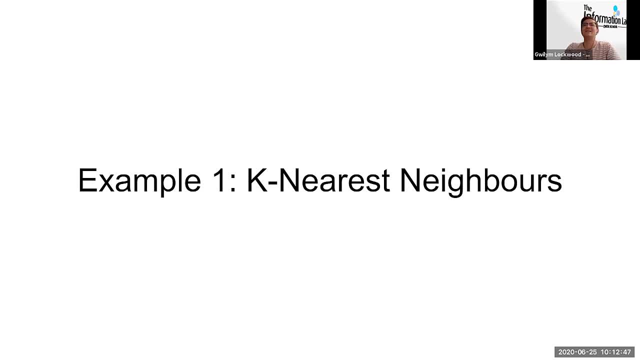 But obviously we're using feature scale measures rather than the actual values you used to, because we don't want to accidentally distort the classification of this. Now, if you're anything Like me or anything like the vast majority of my colleagues or the vast majority of people I've ever met, what you've just heard was probably something a bit like this: 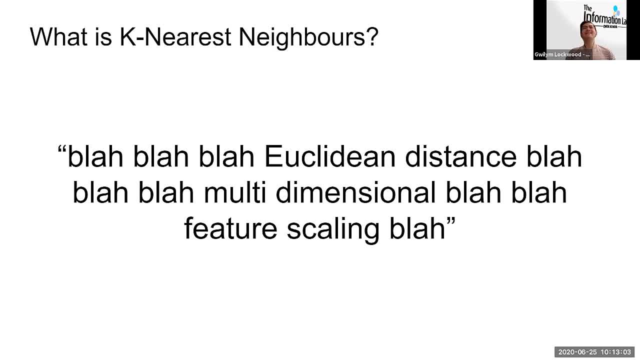 And this is a serious bugbear of mine- Stats and math explanations go from basic to almost patronizingly basic to incredibly complicated instantly, without passing through basic plus intermediate, advanced and so on along the way. So forget everything you just heard. You don't know anything about K nearest neighbors. 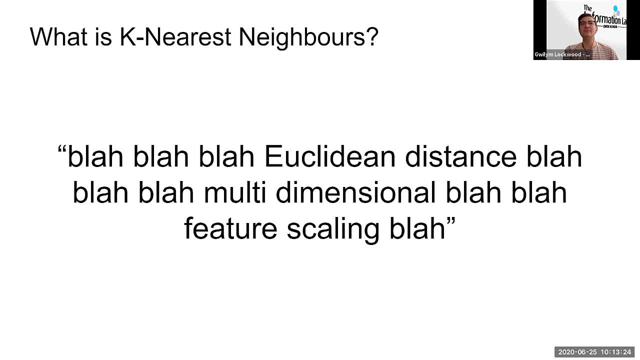 But you do know this. You are in a factory and you are responsible for making machines. It takes quite a while to build the machines, And once you've built them, you've got to test them. Now, testing the machines is also a long and expensive process, because you want to really make sure that they're not going to break. 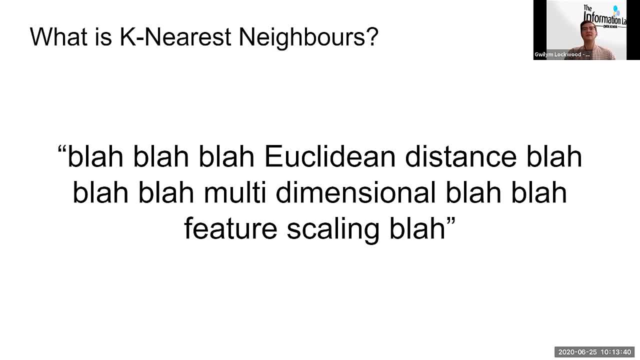 They can handle being run at full performance before you sell it to the customers, And so you want to catch problematic machines and fix them before they go to test, because otherwise you'll waste a lot of time and you'll waste a lot of money. One way of doing this is to compare machines that are currently in production to other machines that you've built before. 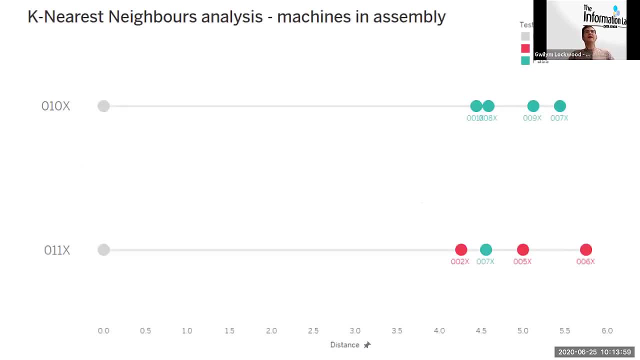 And you can do that with a graph a bit like this. So here's machine numbers 10x and 11x. They're in the factory and they haven't been tested yet. We're in the middle of building them. We were basically just finished. 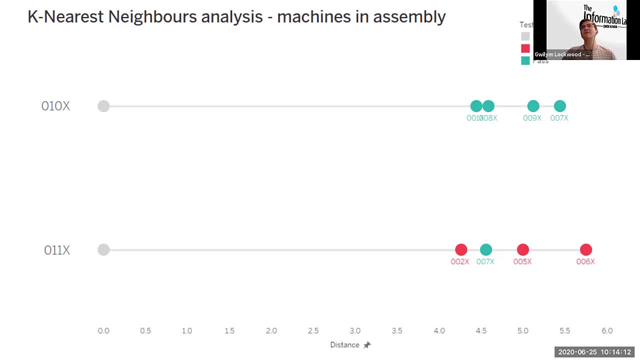 10x is quite similar to machines 1,, 8,, 9 and 7.. All of those machines passed the test and they were sold to our customers just fine. 11x Is a bit more like 2x, 7x, 5x and 6x. 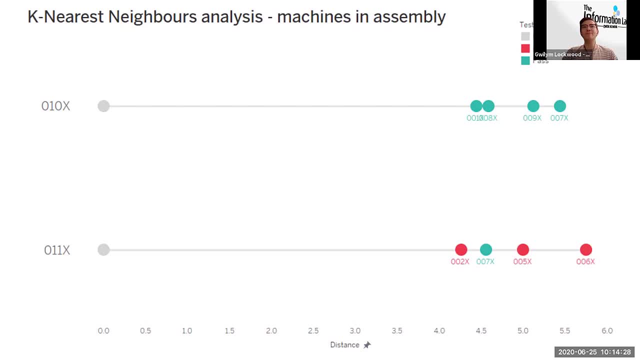 Now three out of those four engines failed the test and they had to be rebuilt before we could sell them. Now I'm looking at that and I'm worried about 11x. It looks like it might fail test, So I want to maybe take it offline. 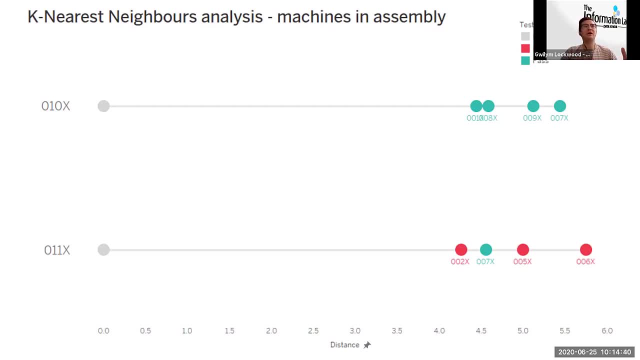 I want to take it out of the production line, adjust a few things, investigate what makes it similar to 2x, 5x and 6x, And maybe fix those problems before the test process tells me. Now, this is something that you can read and understand without having to know everything about how Knows Neighbors analysis works. 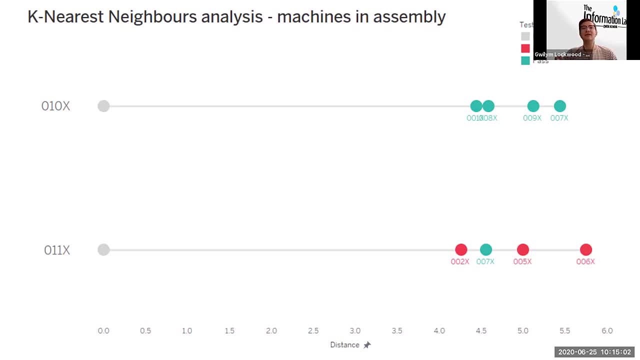 All you need to know is that the distance on the x-axis is a measure of how similar the machines in production are to machines that we've made before, And the closer the machine, the more similar it is, And for many of your users, this is enough. 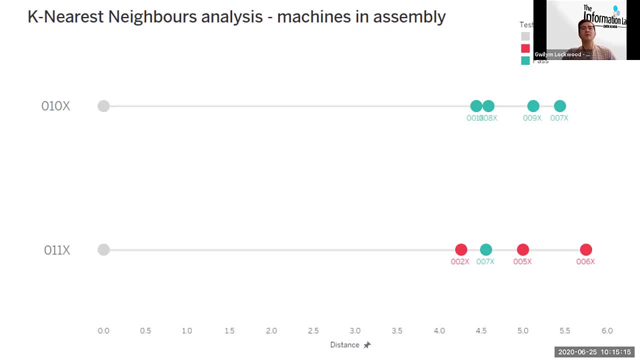 You've done the statistical analysis in the background and you've presented what's important, which is the fact that 11x looks like some of the machines that have failed in the past. That means we probably want to have another look at how 11x is configured before we send it to test. 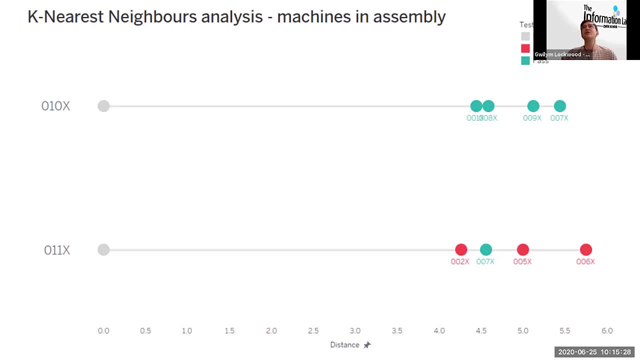 That's all we need to convey in the first place. That's all we need. That's all we need to show to help people in the factory make decisions. We didn't actually need to go into how Knows Neighbors works or how we took hundreds of variables from our manufacturing data and scaled them and put them through an algorithm. 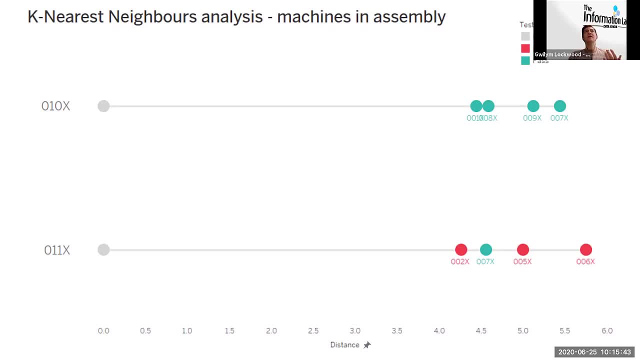 And this is where it gets frustrating as a data visualization professional that you'll get clients saying, oh, we're using Knows Neighbors, But I think people don't understand that, So we'll have to. We'll have to do data literacy first. 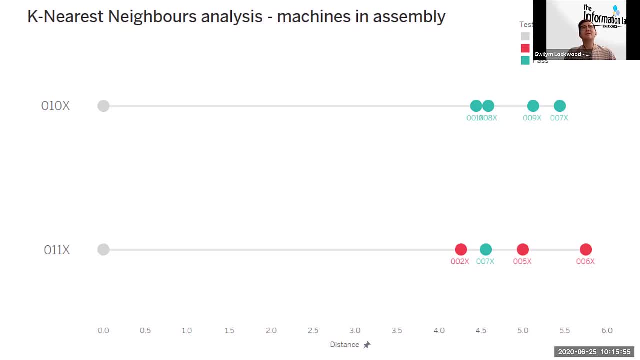 You don't have to understand stats concepts. You don't have to understand Knows Neighbors analysis to understand what's being shown in this chart. But this is a jumping off point for extra data literacy and numeracy training. So if people do want to know more, then that's great. 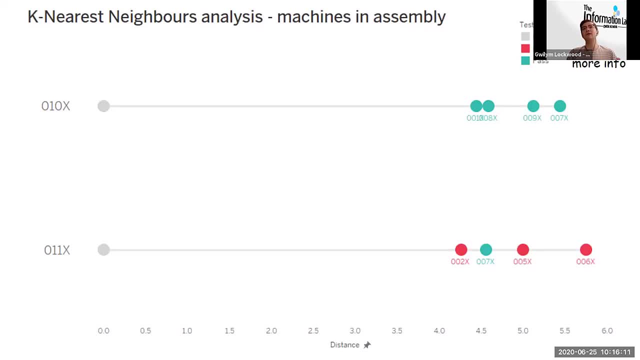 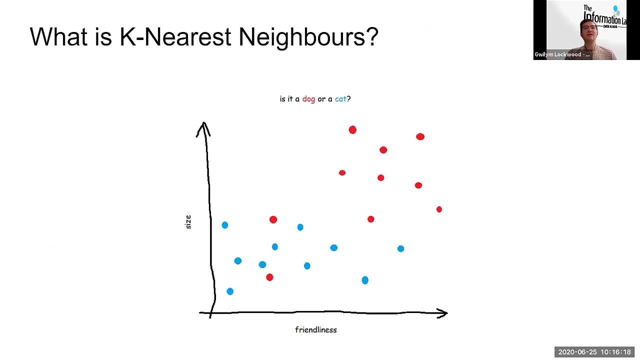 So something I've done before quite often is include a how does this work kind of link to some more resources that people can read for information about the analysis. And I use data visualization in these explanations too, Because, well, stats concept just makes so much more sense when you put them on a graph. 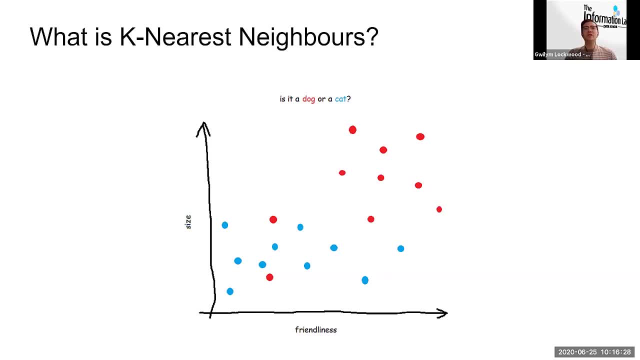 And I also try to use a more interesting, more general data set to make things more intuitive. So obviously people care about their work, but I find it helps to move the topic away from work so that people can see the stats process independently. It also makes it easier for people to ask questions and to explore how it works without worrying that it looks like they suck at their job if they're asking me how something works or asking for clarification. 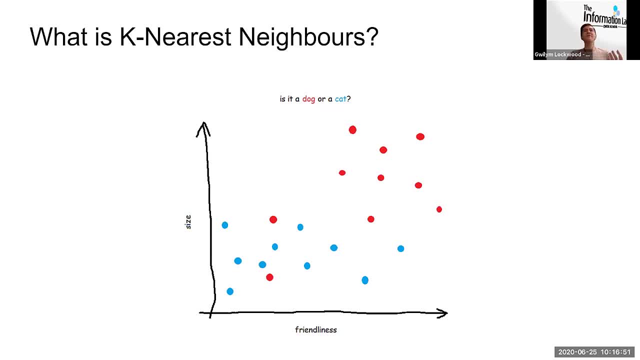 So let's take cats and dogs, for example. You know, I reckon you can tell if something's a cat or a dog easily just by knowing how big it is and just by knowing how friendly it is. But after many years of research and many complicated statistical procedures, I have clustered cats and dogs into 10 distinct types each. 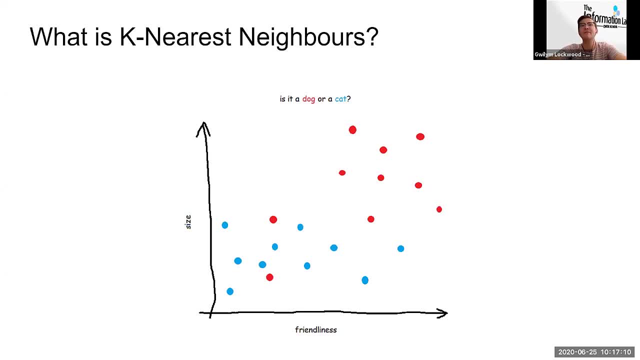 And I've used some advanced graphics software here to plot them on a two-dimensional graph. Red dots are dogs and blue dogs are cats. In general, dogs are bigger and they're more friendly than cats, although there's always exceptions, But for the most part you can tell. 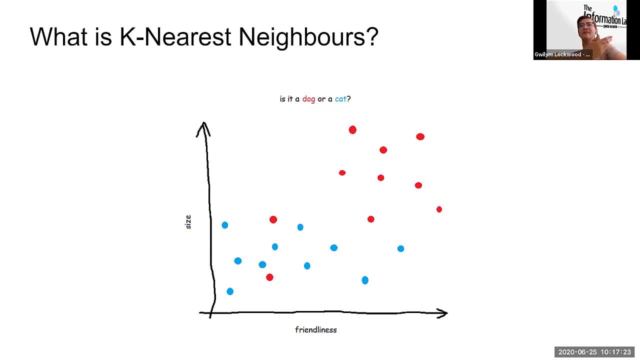 You can probably decide if something's a dog or a cat pretty accurately just with these two variables. A third variable, like aversion to water, would make it even easier, but that would just be a lot harder to draw. So I've got this theory about cats and dogs and the next thing I know, my friend calls me. 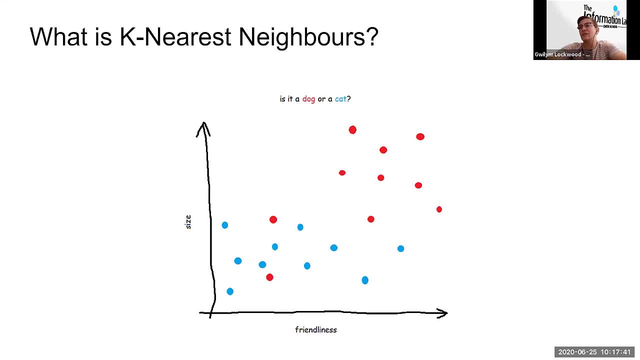 There's some kind of animal in his kitchen and he doesn't know if it's a cat or a dog because he's useless at telling animals apart. So I ask him how big the animal is and how friendly it is. Ideally it's a Z score compared to a normally distributed set of other animals. 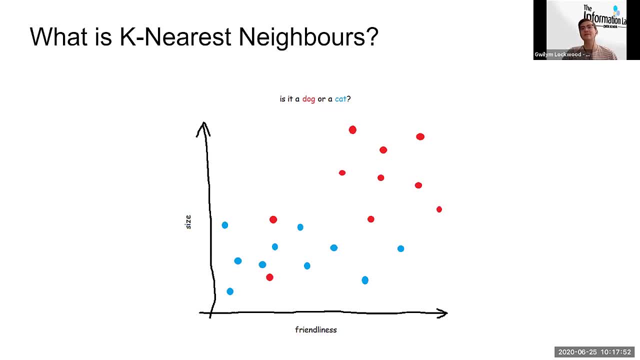 But I'll accept a relative rating if he doesn't have time to go out and do all the sampling. So he tells me it's pretty small and it's not very friendly. Now I've drawn this mystery animal on my graph of cats and dogs by size and friendliness. 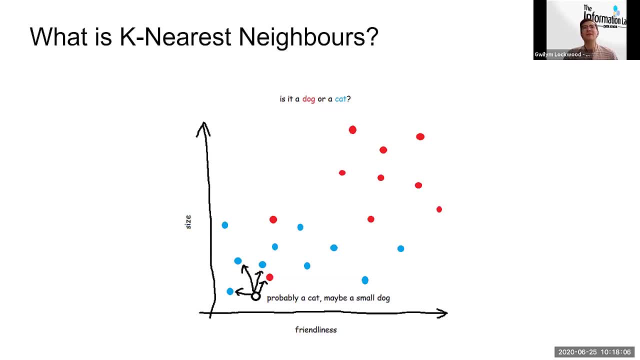 It's the white dot in the bottom left. I don't know what this animal is, but I can make a guess based on what the closest other animals are. If I look at the distance between the mystery animal and the four nearest neighbors on the graph, I can see three cats close by and one dog close by. 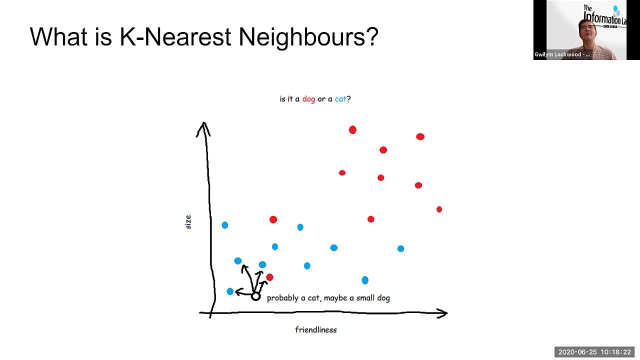 As most of this animal is, I can see that it's not very friendly. If I look at this animal's nearest neighbors are cats. then I can tell my mate that it's probably a cat, maybe a small dog. As I tell him that, he tells me that there's another animal in his kitchen and this time it's really big and it's really friendly. 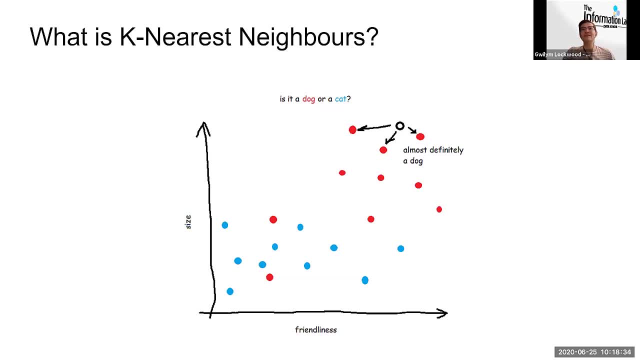 So I plot it on the cats or dogs K&N graph again and I can see that all of its closest neighbors are dogs. It doesn't matter if I set K to 2 or 3 or 4 or 8. It doesn't matter how many nearest neighbors I'm looking at. 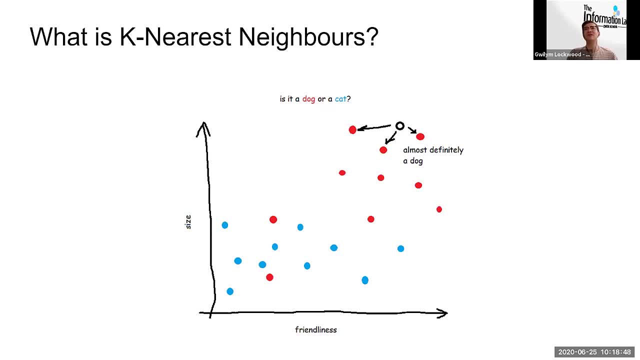 I have to go quite a long way to find a neighbor for this guy. that's not a dog, So it's almost definitely a dog, And my friend says he's getting the hang of it now. And then a third animal walks in and he's stumped. 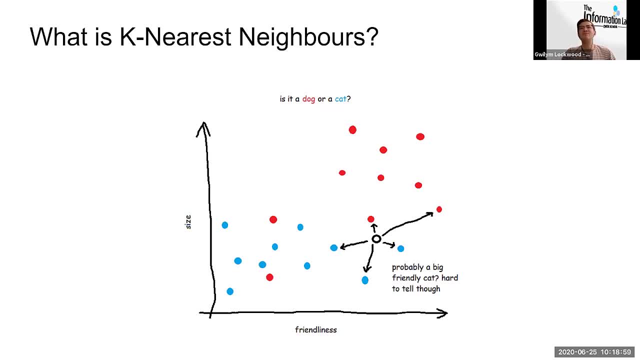 This animal is sort of on the smaller side of medium size and it's pretty friendly. So the K&N on this animal is quite unclear. If we look at its five nearest neighbors, there's two dogs and three cats, And so maybe it's a big, friendly cat, I reckon. 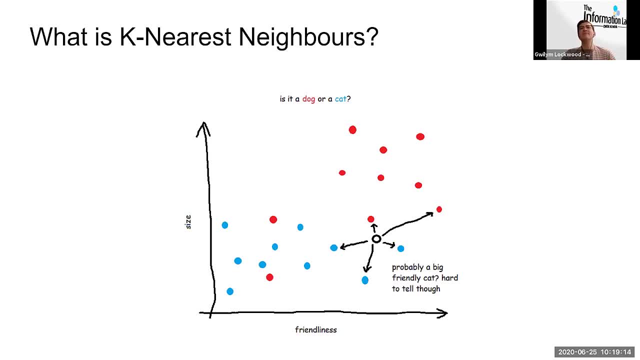 It could also be a small-ish dog. It's hard to tell. So at this point my two variable taxonomy of dogs And cats is starting to look a little inadequate, So I might have to reconsider the whole thing and add a third variable after all. 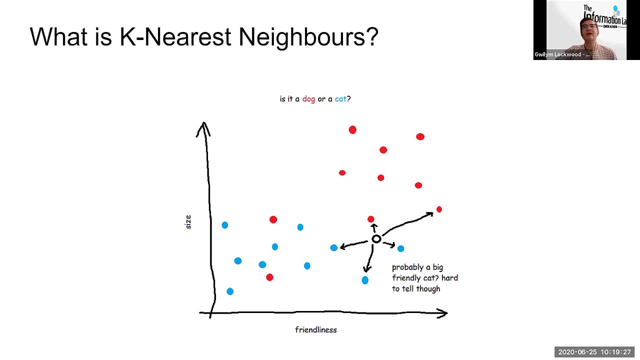 But while I'm doing that, I'm hearing a scream from the other end of the phone. A fourth animal has walked into my friend's kitchen and something's gone terribly wrong, And it's exactly as I feared. He's tried to use the cats and dogs K&N analysis on a data point that's totally out of scope. 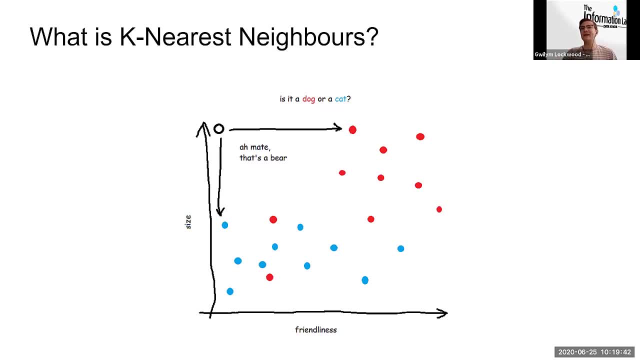 He's seen an animal that's really big and really unfriendly And the K&N analysis has told him that it could be a dog or a cat, but it's probably a dog And the problem is it's actually a cat, It's actually a bear. 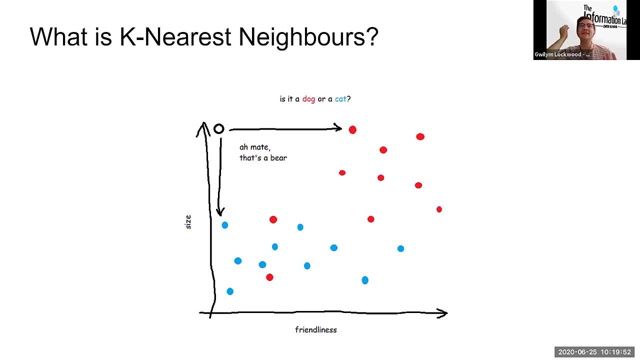 And the K&N analysis can't detect that it's a bear because we don't have any bears in the input data- Rookie error. So as I hear my friend getting mauled in the background, I start updating my K&N model input data to include some more animals. 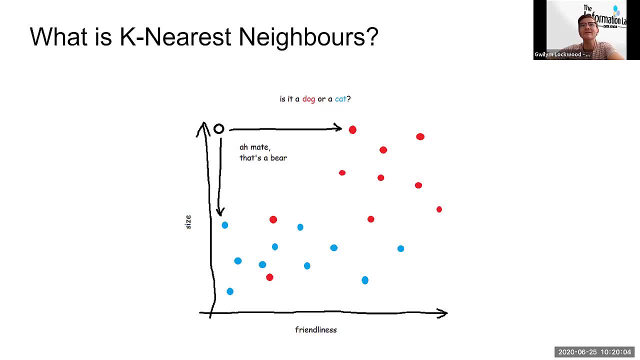 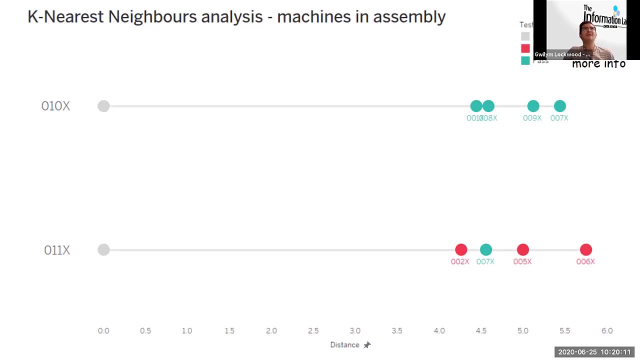 so that this analysis can be deployed at scale at a wider variety of clients. And now we're back at the manufacturing dashboard And the users across the organizations now have a sense of what kind of analysis and what kind of steps and processes have gone into this simple, understandable graphic, without being too overwhelmed. 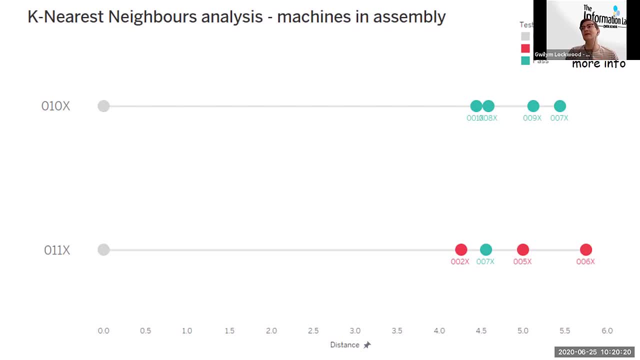 So They can see. they can always see and ask more about the stats and the process for the manufacturing data They can investigate. that I would offer to. that's the point where I'd be proactive and offer to run extra sessions for the people who are interested. 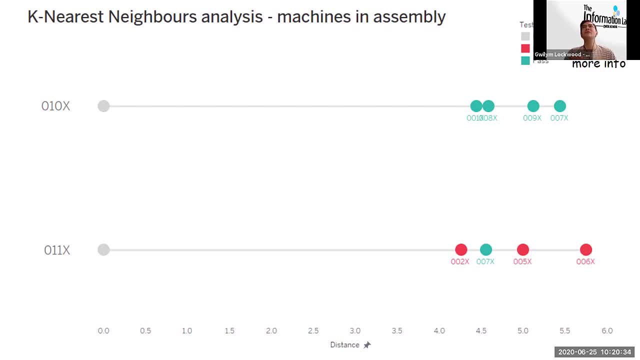 But for the vast majority of people this is enough, And the point is, it's enough for them to do their jobs and make decisions and use data and data visualization Like from data fears to numeracy, rather than the other way around. I'll show you another example from the same kind of manufacturing data using Z scores. 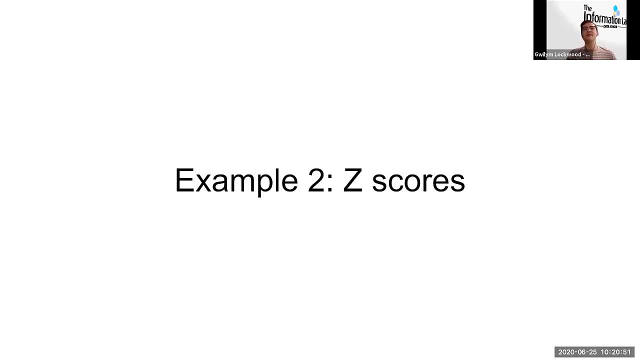 Z scores aren't as complicated as K nearest neighbors analysis, but I'll just define it quickly. Anyway, a Z score is a standardized score which shows the difference between a particular value and the population mean all divided by the population. standard deviation. 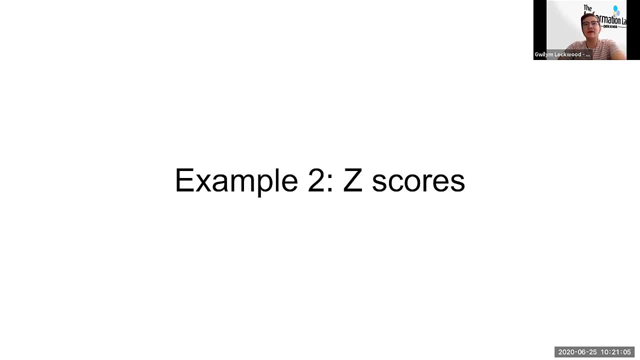 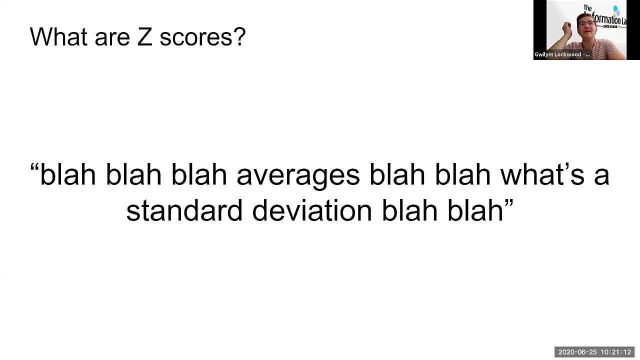 which means that a Z score shows the difference above or below the mean in terms of standard deviations. And again, that probably sounded a bit like this And it's so frustrating. It's infuriating because statistical explanations like this are so much more complicated. 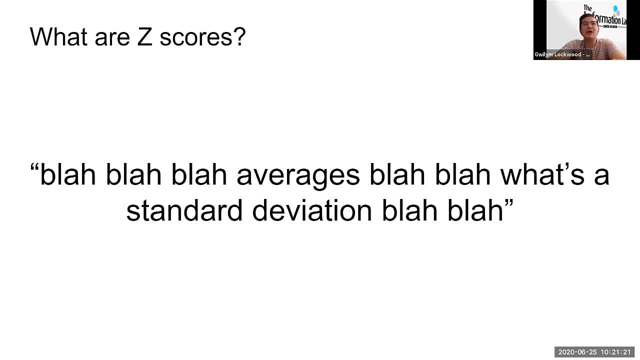 And it's so frustrating that they need to be. Conceptually, a z-score is really easy to describe. it's just like saying: how much is something, but relatively speaking, rather than absolutely speaking, just how much is something relatively speaking? So again, let's forget about z-scores for now. This time you work. 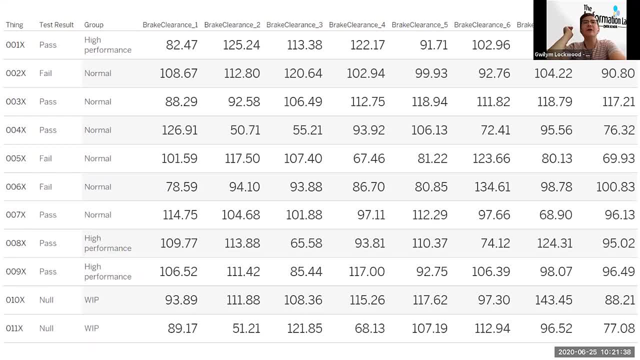 on the machines in the factory. Let's say that these machines are really, really fancy cars. What you do is you adjust the brake pads so that they align properly with the wheels, So like- yeah, if you imagine, like a brake pad that presses up against the wheel to cause a load of friction to. 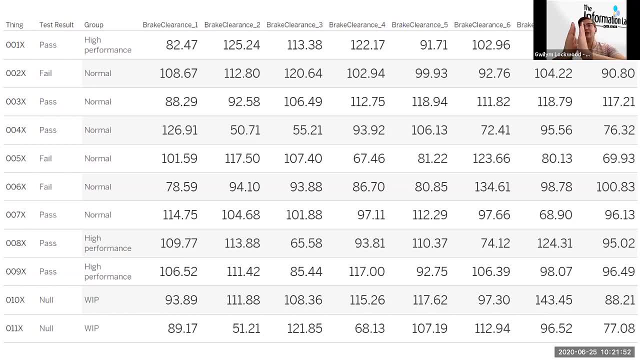 slow the wheel down. You want the pad to be the same. I'm just going to gesture like this instead trying to work it out on zoom. yeah, there we are. You want the pad to be the same distance from the wheel across the whole pad, rather than, like you don't want it to be set at an angle so that the 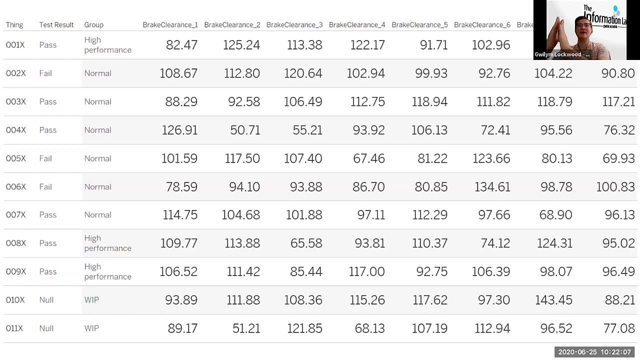 pad doesn't fully touch the wheel when you hit the brakes. You want it to be sort of set as parallel as possible so that when it depresses the majority, as much of the pad as possible touches the wheel The same amount of possible when you hit the brakes. So what you do is you measure the 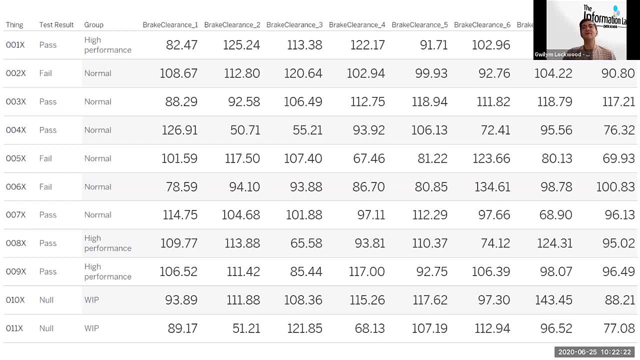 clearance between the brake pad and the wheel at eight different locations to check that it's consistent. Now, some of these values are higher than others, and you don't mind a bit of variation, but what you want to know is if things are relatively higher or lower than normal. 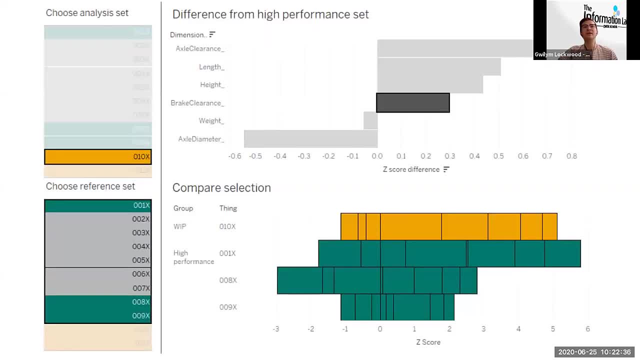 across all of these brake clearance measurements. I mean, you can, we can use z-scores for that. So let's take machine 10x, which was the the one that we were pretty happy about in the KNN analysis earlier. Let's compare 10x to the high performance machines, the high performance cars. 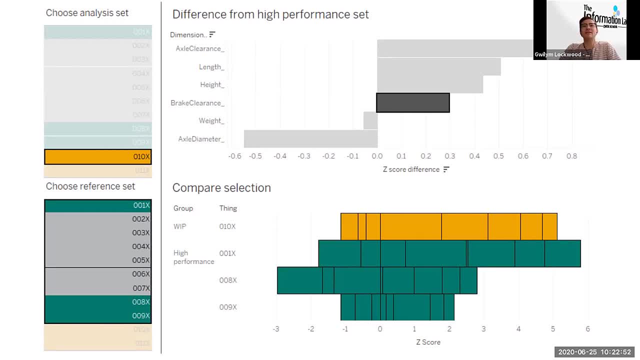 So 1x, 8x and 9x. they all perform really, really well in the test, So ideally we want all machines to look like 1,, 8 and 9x. The stacked bar chart at the bottom right: this shows the, the z-scores. 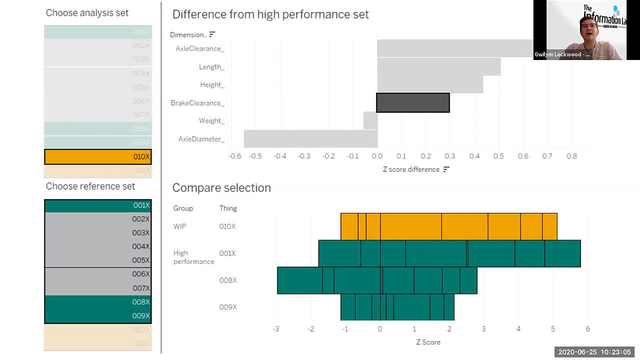 for each brake clearance measurement. for 10x in yellow and the high performance engines in green, We can see that they're quite similarly distributed. So most of 10x's z-scores are above zero, somewhere in the 0.5 to 1 range, and you could probably say the same thing for for 1x. There's a couple of z-scores. 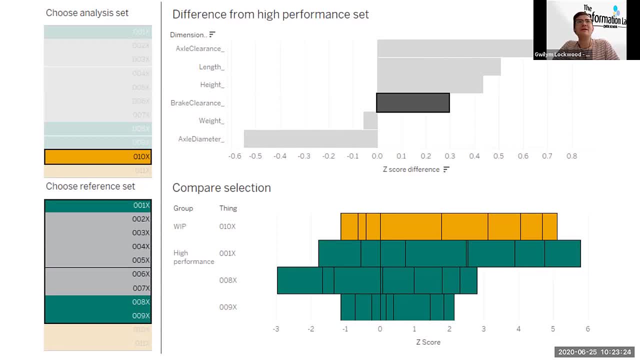 that are about maybe one and a half that. that looks like the biggest z-score for 10x. Similarly, the biggest z-score for 1x looks like it's about that. looks like it's about 1.6, but yeah, most of them are in the 0.5 to 1 range. This is like a nice trick, So we're not comparing. 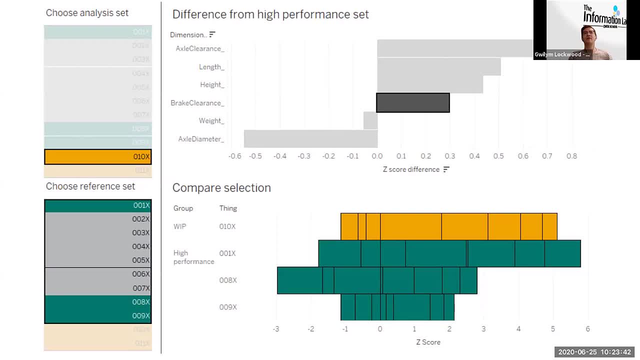 we're not just comparing 10x to the high performance machines. we're showing that when it like we're comparing it to the whole reference set. So 10x and the high performance machines differ from average in about the same way. So we're comparing the difference from average for. 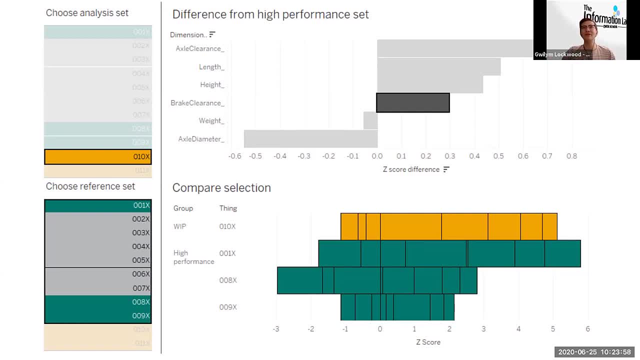 10x and the difference from average for 1x, and showing that they differ from average in a similar way. And that's what's shown in the grey bar chart at the top. So the average z-score difference between 10x and the high performance engines is only 0.3.. So what that is is, if you imagine, 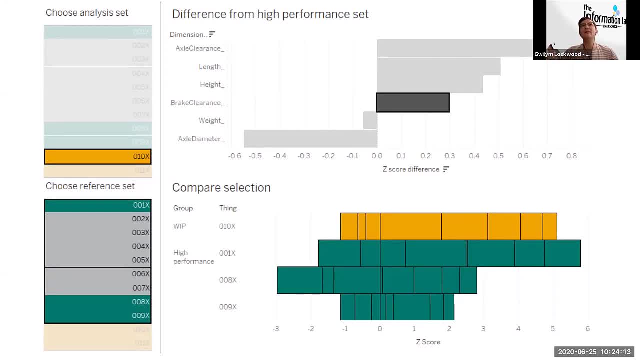 if you take the average, the average z-score for all the bars in yellow in the bottom, and try and picture where that is on the on the chart, which is probably somewhere around- if you can gesture with my mouse here, it's probably. the average is probably somewhere. 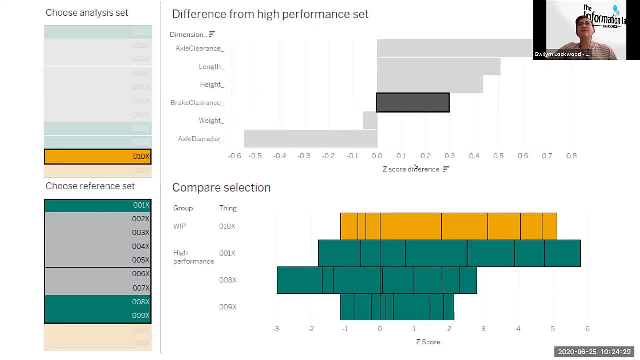 around here I'd say: And then you're taking, the average is for all the, all the green ones. so the average is probably around 0,, maybe 0.2, 0.3.. Then we're looking at the difference in. 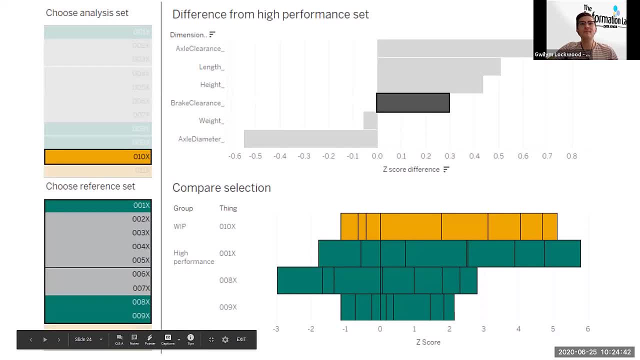 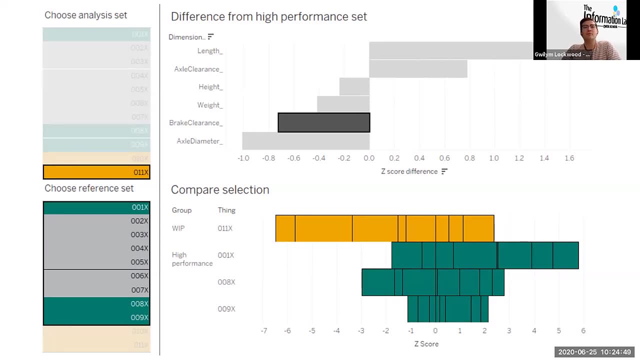 those averages, which is about 0.3.. So let's compare that with 11x, where the average z-score difference between 11x and the high performance engines is minus 0.8.. That means that the z-scores for 11x's brake clearances are 0.7 lower than the the z-scores 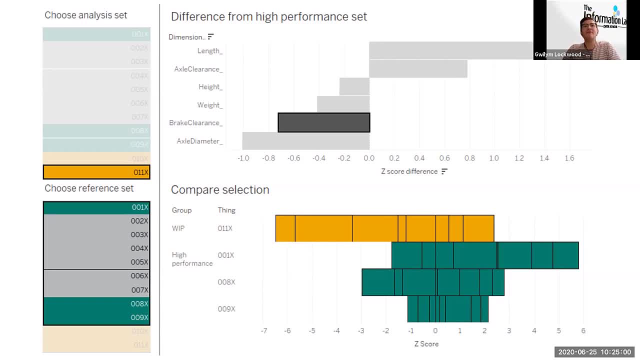 for, sorry, 0.8, lower than the, the z-scores for the high performance machines, And we can see that this in the in the the bottom chart. So do you notice how the stack bars for 11x are mostly? 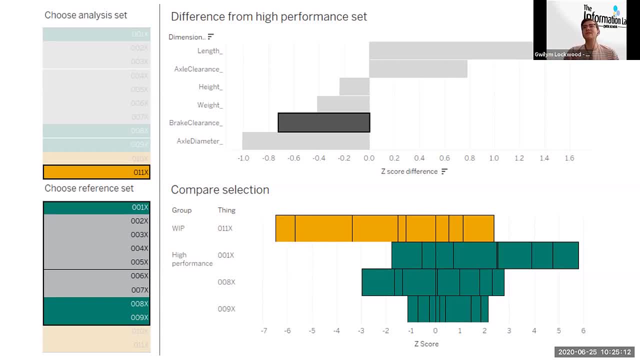 negative and relatively wide as well. So, in short, this is telling us that 11x just doesn't look like high performance machines when it comes to brake clearances. Based on the chart above, it looks like it does look quite a lot like the high performance machines when we look at height, but for brake 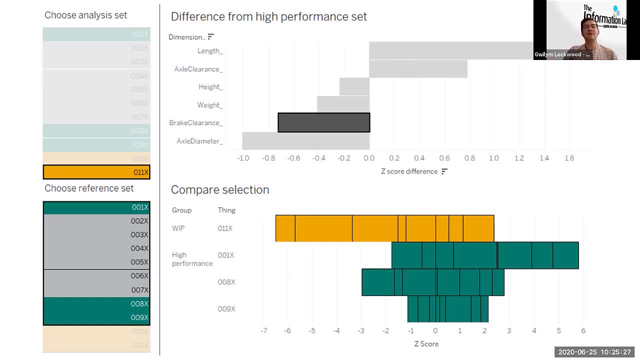 clearances not so much, So 11x doesn't look like them in terms of brake clearances, 10x does, and that gives us the ability to look at exactly where. And again, if people aren't fully fluent at z-scores yet, this is a great opportunity for doing some data literacy and numeracy development. 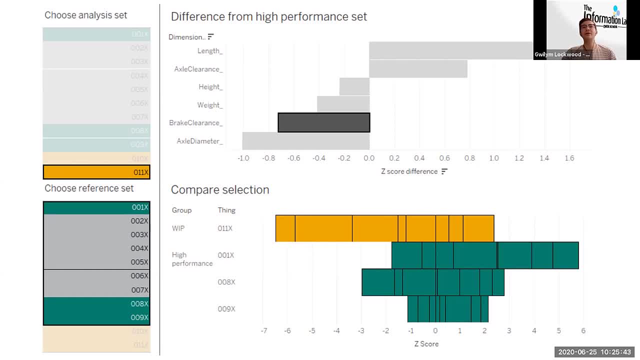 either as a click for more info- kind of thing that we saw last time- or, in this case, where the data utilization itself is quite complicated, You could run a user training session to show people how you've designed it and how they can get information from it. We do this sometimes with 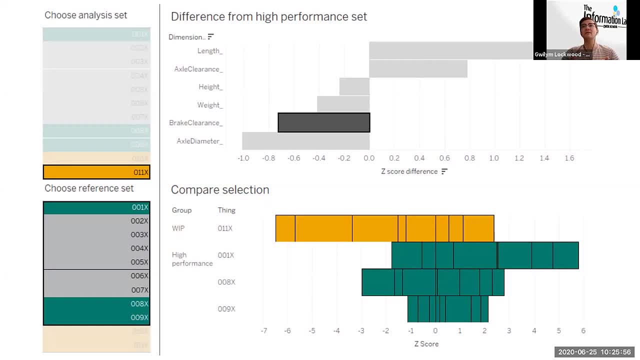 with different clients, when, if we've spent a long time creating dashboards that are quite complicated like this one, we'll, when we announce the, the, the dashboard, we won't just say, hey, there's a new thing up, go explore, We'll, we'll, we'll send out an email. 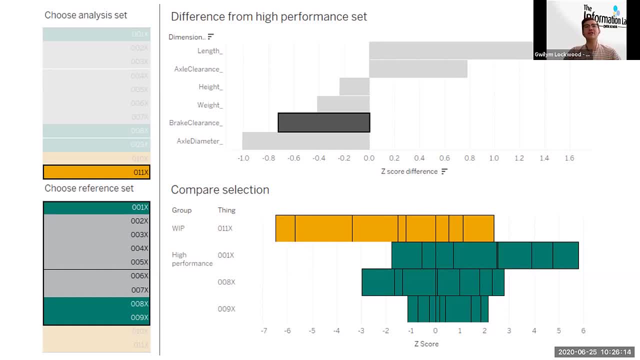 we'll announce it on the internal Slack channel or whatever communication platform we're using, and also schedule in some sessions. We'll we'll do some. hey, this is how you can use this dashboard for your analysis. Let's have a quick half hour explanation session with. 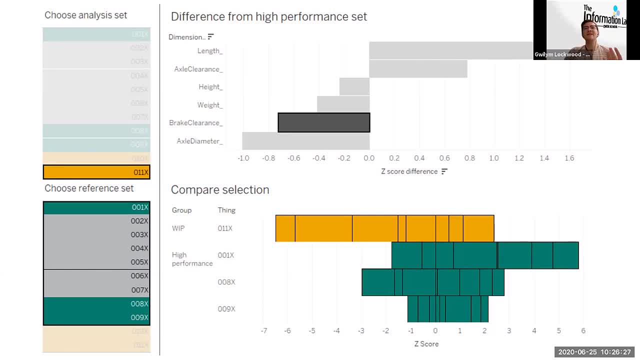 with people And that that often works really well. So again, z-scores are totally intuitive once you've seen them in the right context. So when I'm doing these training sessions, I often use an example with with my height and where I've lived. So this is, this is me, This is. 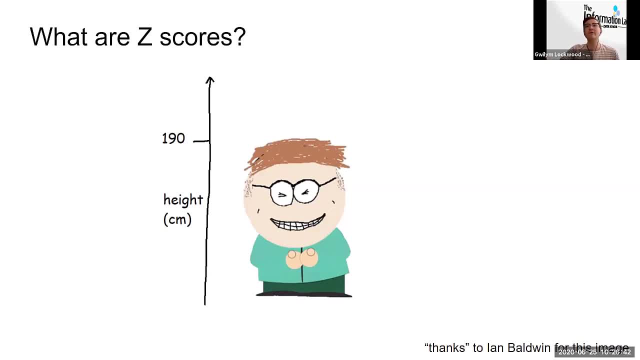 a better pre-COVID-19 haircut than I have right now, which I've just been doing in the bathroom. I'm 1.90 in height, which is about 6'2, 6'3.. And that's a, that's just a fixed property. It's. 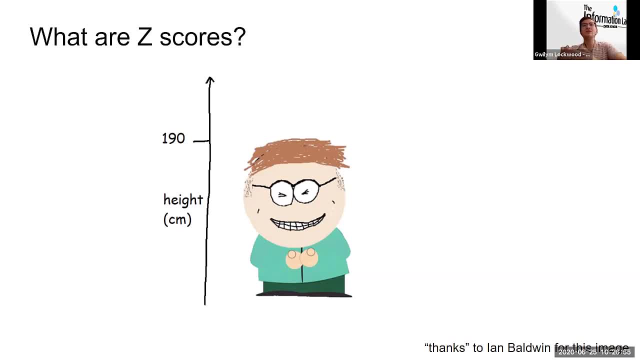 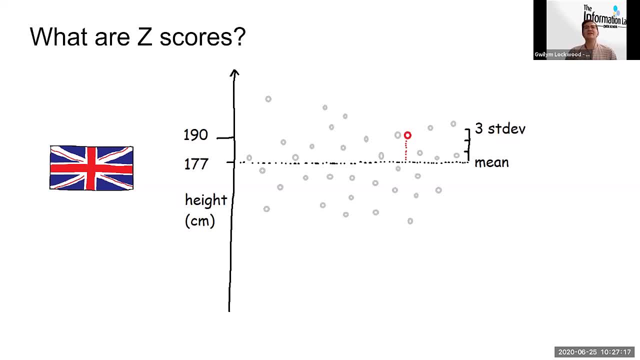 so I don't stand out as particularly big. I don't. I don't. I've never had to go to any kind of specialist clothes shops, and I'm never the tallest person in a room, And that's not just because I'm never in a room with anyone at the moment either. I couldn't find the. I couldn't. 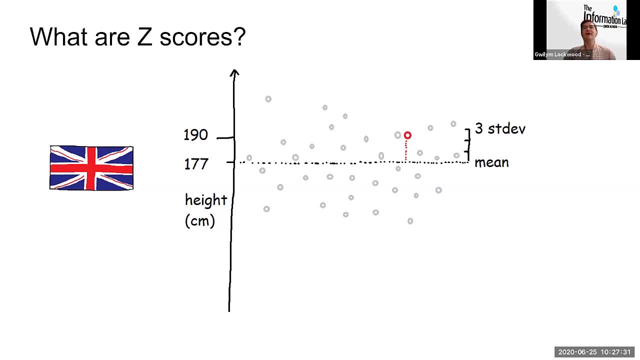 find the UK's male heights standard deviation or anywhere online, which, yeah, it was just surprising. I'd have thought that with something as as frequently measured as height and as frequently used to explain normal distributions as height, you'd think you'd be able to find standard. 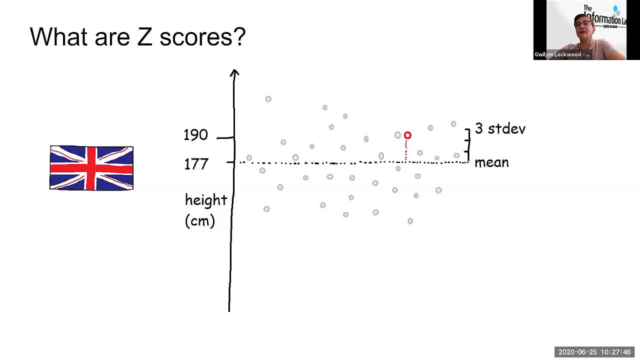 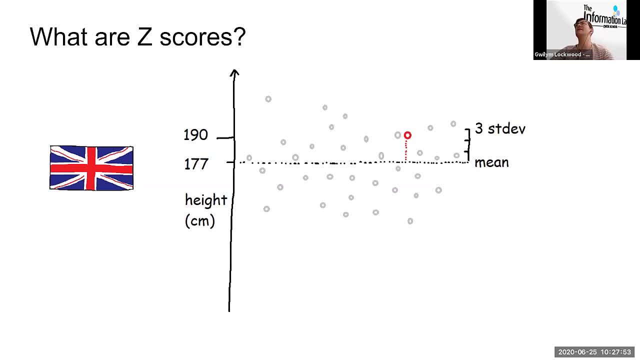 some like reputable, actual standard deviations of height for men and women in the UK? please let me know. I'd love to. I'd love to see a good data set. Anyway, as a guess, I reckon I've got a Z score for height of about two, which means relatively tall, but not really massively tall. However, when I lived in Japan, that was a completely different story. I'm exactly the same height, but the perception of how tall I was was completely different. So I'd say that I was about three and a half inches taller than the average male height in. 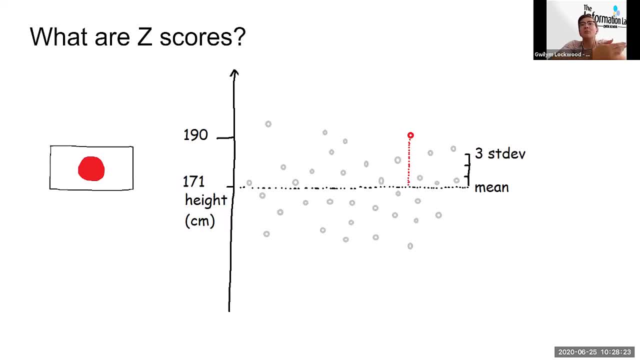 the UK And I could feel that higher Z score I would. I normally was the tallest person in the room in Japan and it was hard to find clothes that fit. So even like a lot of I'd go to Japan's like H&M or Uniqlo or whatever And the the largest t-shirt sizes I could find that was still. 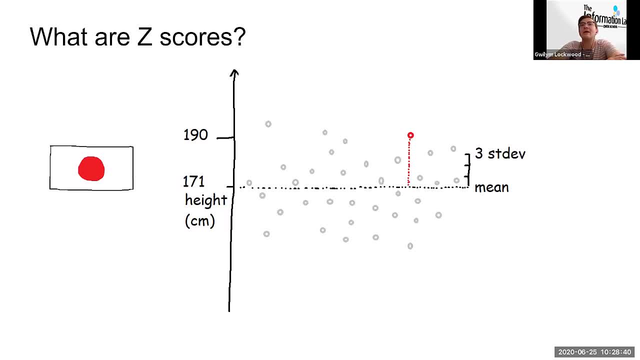 pretty, pretty tight on them And I, so I reckon I probably had a height Z score of about three and a half, maybe four, in Japan. And then after that I moved to the Netherlands, and in the Netherlands everyone's a giant and I was pretty much average, So I was. I was about eight centimeters. 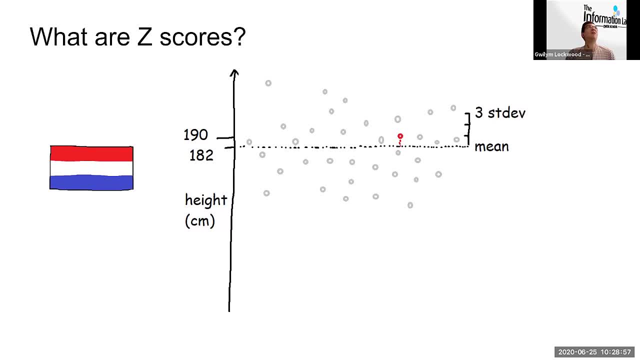 taller than the average height, which is probably only like half to one standard deviation or so. So a Z score of one basically just means that I'm a bit taller than average, but pretty much just in the middle, And that there were, like there were, a lot of times that I was actually the shortest. 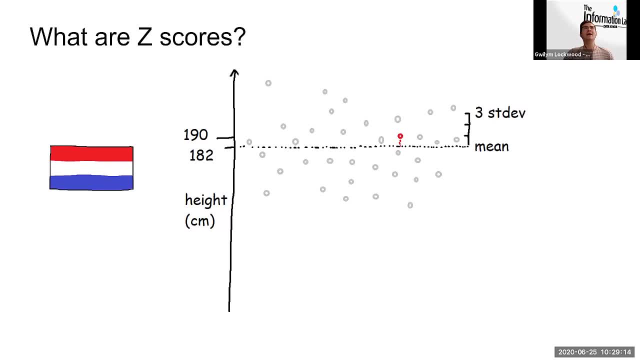 person in the room And some of the times I was the shortest person in the room And some of the times I was the shortest person in the room And some of the times I was the shortest person in the room. So that's something that never happened to me in the UK would be that like I'd go to a, I'd go to a. 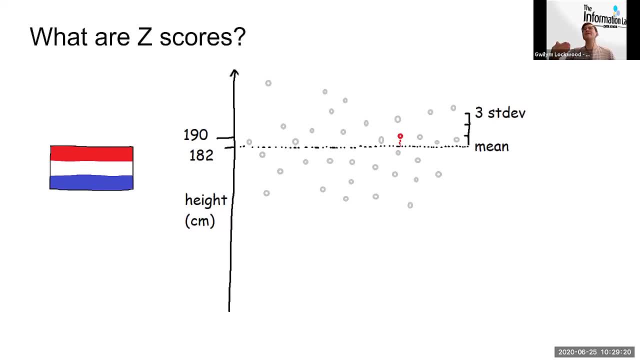 gig in the Netherlands and I'd be in the second row And the three guys standing in front of me were all like six foot eight or two meters five or something like that, And I couldn't see at all. That's never happened to me in the UK. It happened to me relatively often in the Netherlands, So Z. 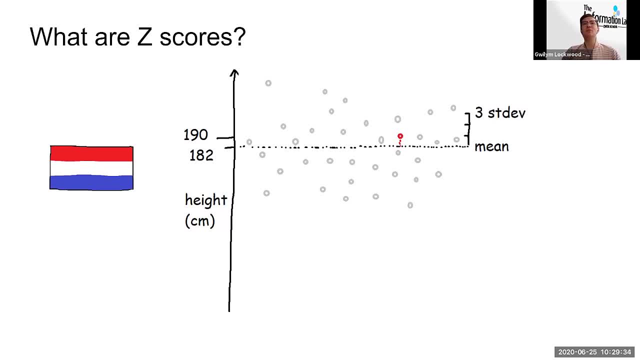 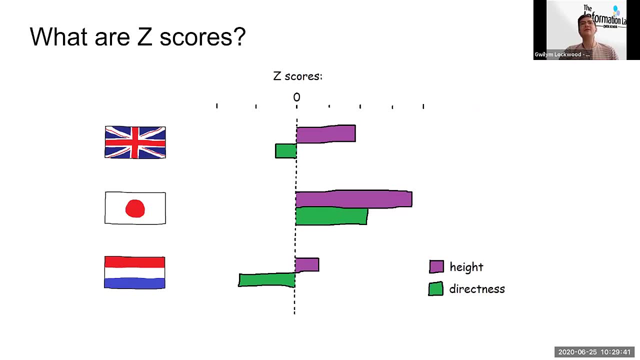 scores are a really good way of consistently measuring how different something is from normal and not relying on its fixed property and making inferences from a fixed property. The best thing is, you're not limited to one unit either, So, for example, I can compare my height in centimeters with my personality as measured in. 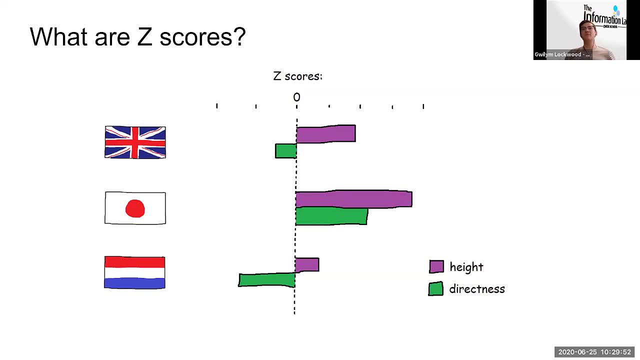 hypothetical units of directness. So in the UK we're not a particularly direct people And I'd say that I'm maybe a little less direct than most Brits are as well. But in Japan, where I found, I found Japanese society really, really indirect, I suddenly felt 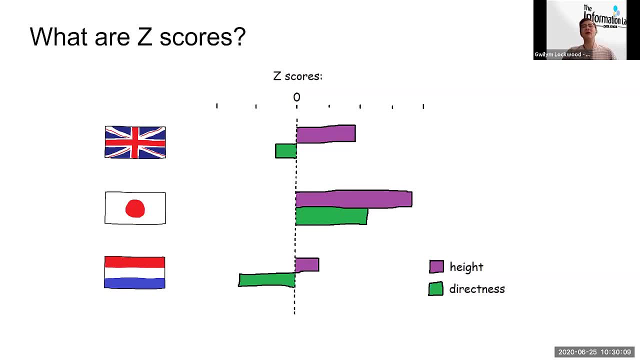 like how Americans do in the UK. where Americans are here, It's like why is no one saying what they think? And then when I was in the UK, I was like why is no one saying what they think? And then when I was in the UK, I was like why is no one saying what they think? 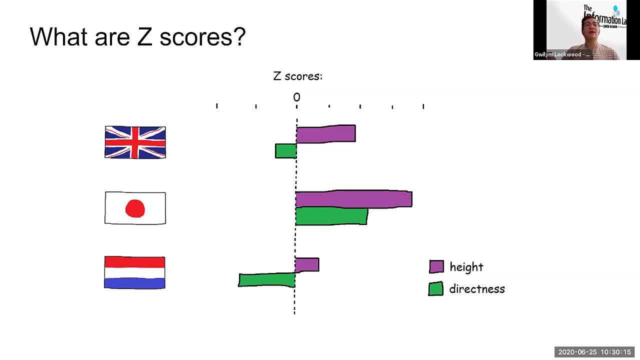 And then when I was in the UK I was like why is no one saying what they think? And then when I moved to the Netherlands, where everybody tells you exactly what they think of you all the time, I felt incredibly indirect and sort of felt like every sentence that I said in the 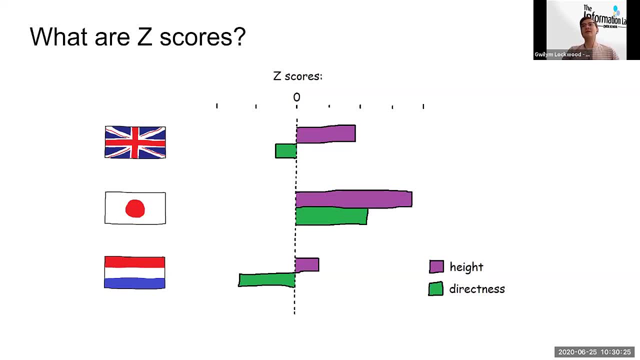 Netherlands was beating around the bush rather than just saying no. I think that this idea is. I think this idea is bad, Let's move on, which is which is the Dutch way of dealing with things Took a little while to adjust to, but it was actually quite refreshing. I liked it. after a 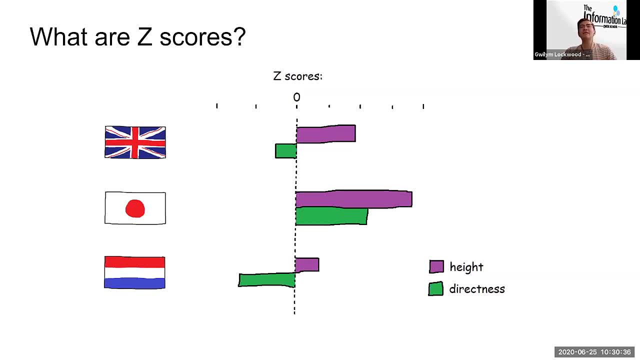 while. But anyway, now I can compare lots of things in lots of ways by expressing it as a relative measure rather than an absolute one, And those relative measures are the ones that are really useful in manufacturing data, and those relative measures can be compared. But I 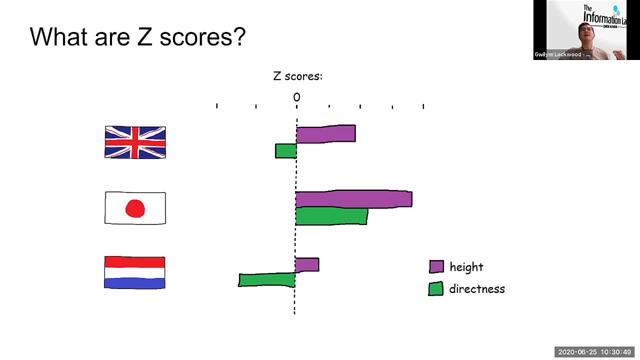 can see from this graph that I stood out more in Japan in terms of height than in terms of directness. That's not a comparison. you can do in centimeters or in units of directness, but you can with Z-scores. So it's great for manufacturing data, because it means that we 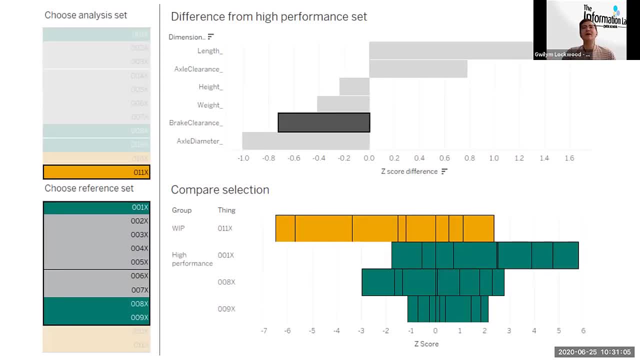 can look at 11X and we can see that it's different from the high performance engines in terms of all the different brake clearances And we should maybe address that And you can go more broadly as well. So, in the actual data that this comes from, the sort of dimension, groups like brake 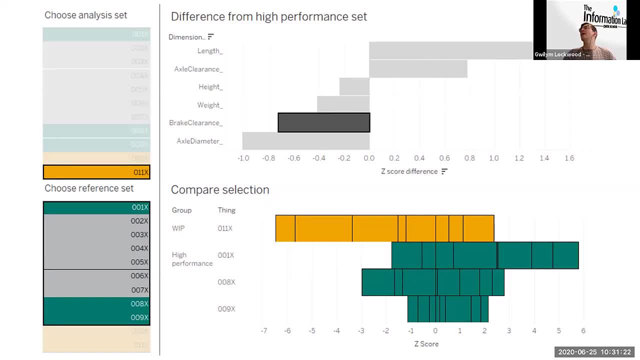 clearances, we use sort of slightly more general kind of performance measures- or sorry, not performance measures, but these slightly more different measures related to different bits of the machine. So if we're talking about one specific part, because it's all related to that, 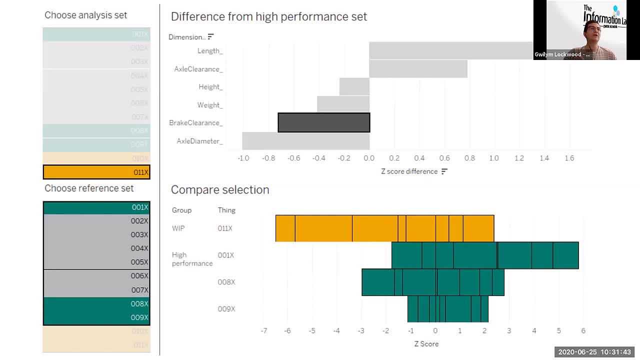 particular part. we'll see that We'll look at the weights of the ball bearings or we'll look at the clearances of different things, And those are obviously measured in very different units, like weights versus distance, And we'll group those all in together in the same group to look at how different this particular 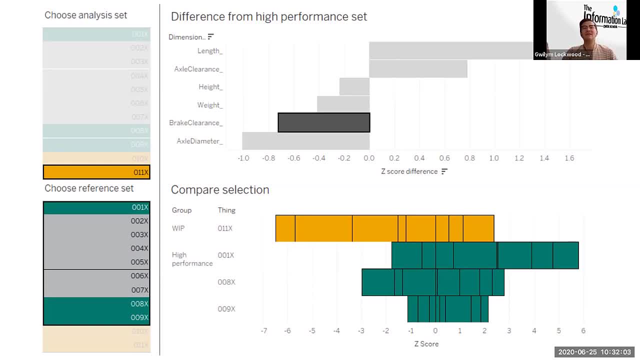 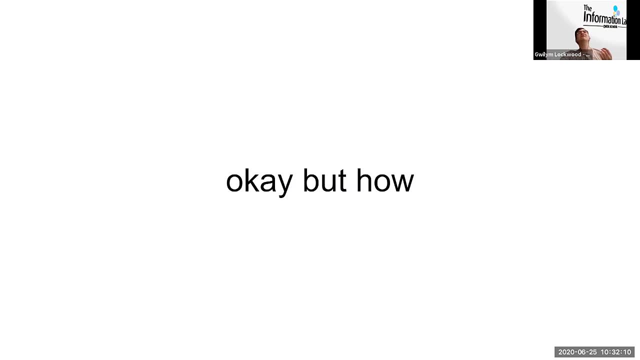 bit of the engine is compared to the rest of the machine or whatever. So, yeah, those are really really useful And okay. so this is the bit at the top where we get to. okay, but how are you going to make Microsoft Paint diagrams for everything all the time? Well, 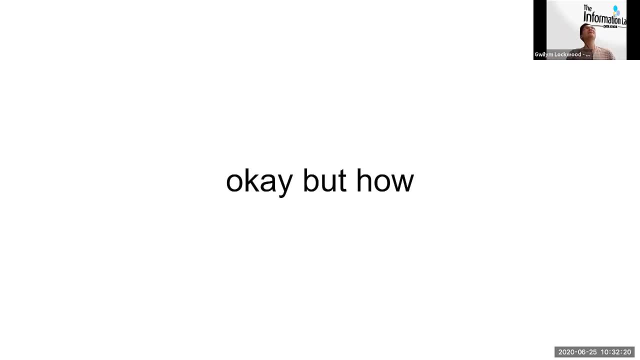 yes, actually It's a bit silly and it feels a bit silly to make these diagrams, but there is a method in the madness. I find that for something like maths and stats, where a lot of people, including myself, feel quite intimidated by it, quite a lot of the time there's something. 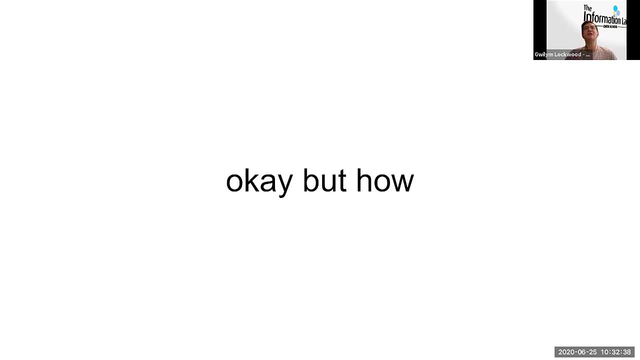 about expressing it in a slightly, deliberately silly way, or a deliberately uncomplicated way, or in an almost deliberately unprofessional way. There's something about that method of expression that makes the whole subject a lot less intimidating. And then, as soon as it feels like something you can laugh at, as soon as it feels like something you can smile at, it feels 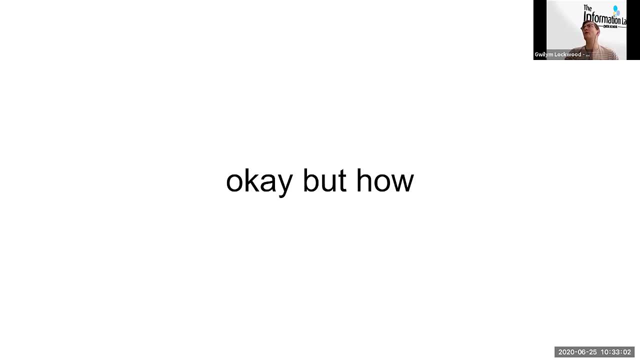 a bit demystified and people can approach it on a more open level, without trying to cover up how we feel intimidated by maths and stats. And it's like I get paid to do this for a living and I still feel quite intimidated by analyses I don't understand right at first as well. So yeah, 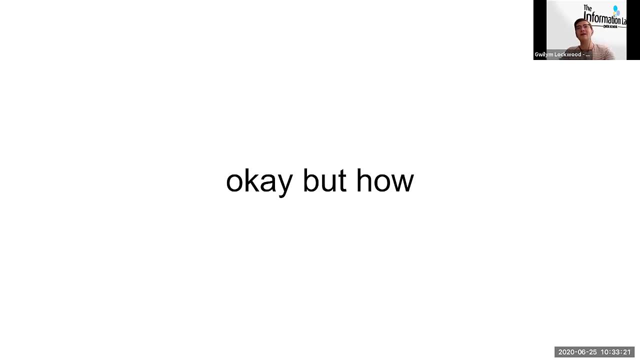 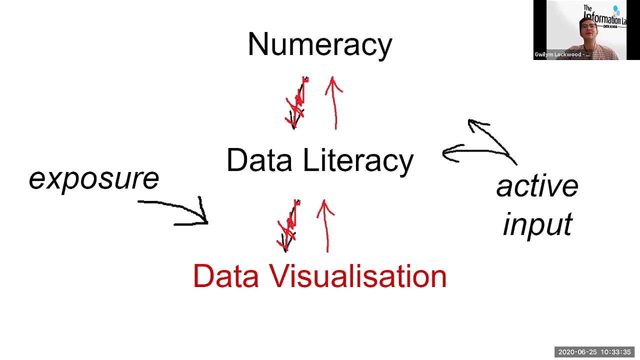 I find that putting things into fun little diagrams helps quite a lot. But yeah, so there's, I'd say there's three main ways of addressing this sort of thing. The first is that, the dedicated training option, So you can tailor numeracy training to the 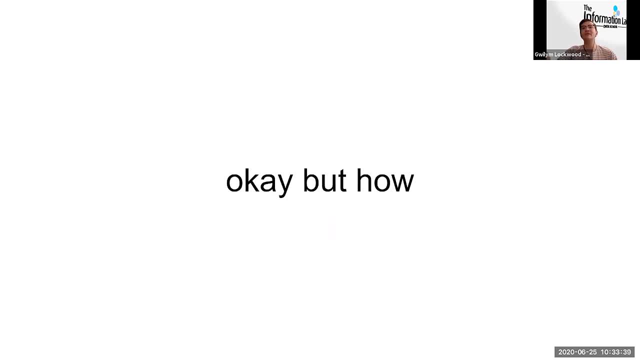 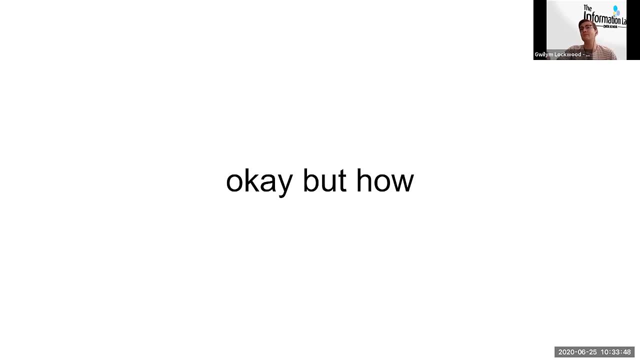 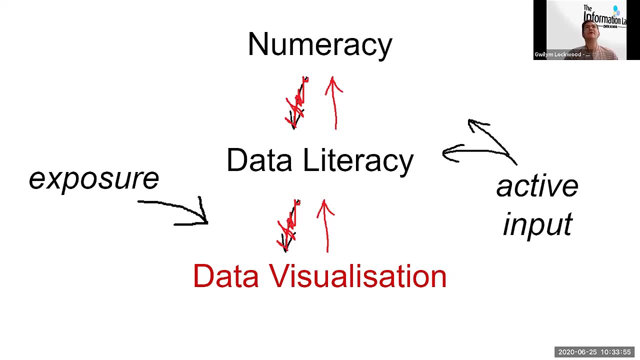 and the human option, which is to make yourself known as a friendly face who's happy to help, and people will just come to you. So, yeah, this is where I see that fitting in with the slide that I presented right at the start. Instead of going from numeracy to data, literacy to data, 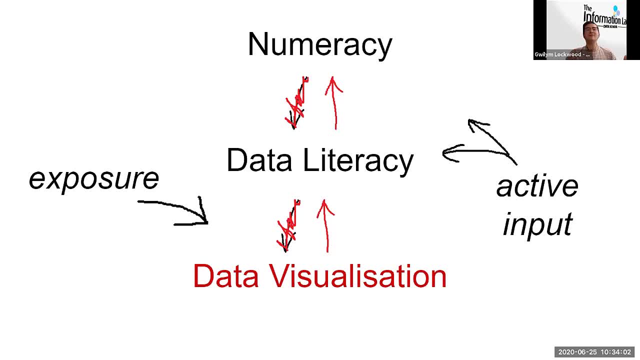 fit. go the other way around, where you can start out with data visualization, because people care about data visualization. You can then use that to bootstrap data literacy and numeracy. So the first thing is the exposure. It's roll out your interesting, roll out your well-designed data. 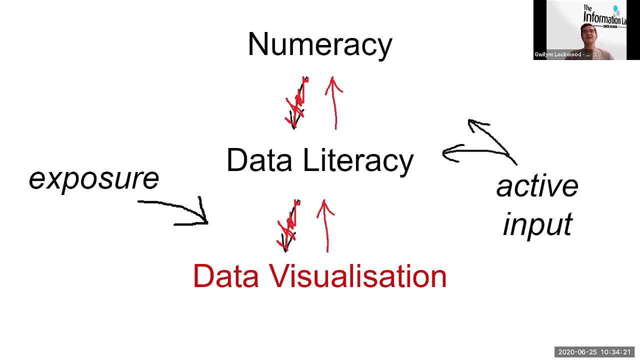 visualizations and watch people interact with it and see what happens. That's the exposure phase And then the three. okay, but how parts? that's the active input phase for data literacy and numeracy And that's where you can see how people have reacted to your data visualization. You can see 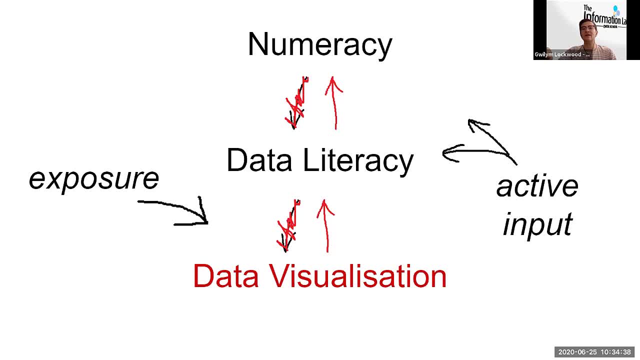 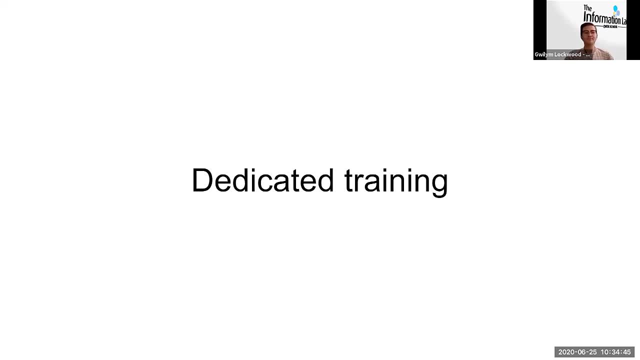 how they're getting on, And then you can proactively scaffold a development and understanding. So yeah, I'd say that's through dedicated training. Like I said earlier, it's not. I rarely find that a one-size-fits-all approach for data literacy, data numeracy, data viz training. 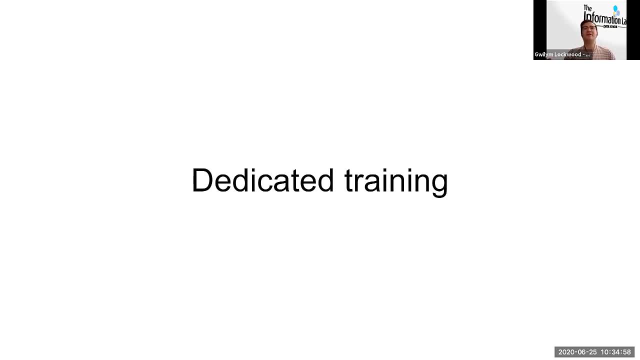 I rarely find that that works, because everyone's coming from a different level, everyone's coming from a different background. When you've got people who people come from degrees in engineering, who sort of go to bed and dream about sales scores when they're working. 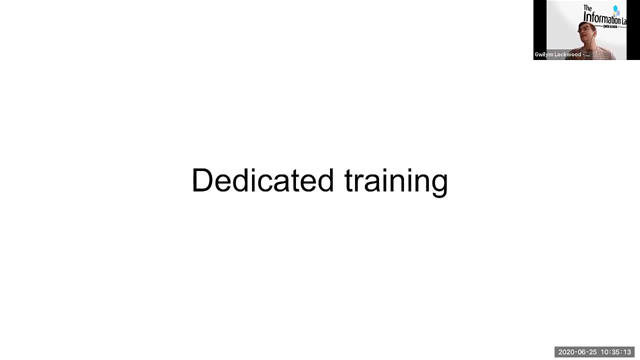 alongside people who, let's say, did humanities degrees and do or trained as marketers, and they're great at their job, but their job doesn't involve maths very much. therefore, these are completely like unfamiliar mathematical concepts to them. But putting those two people in the same training 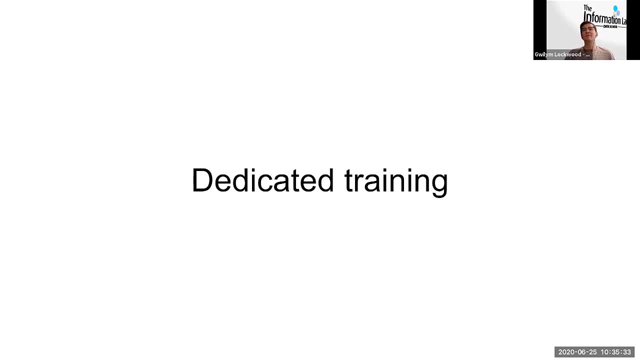 session. one of them's going to be bored, one of them's going to be overwhelmed. It helps to separate people out into smaller groups and tailor it towards them. That also makes it more fun as well, because people will be. I find that people are much more happy to engage with training sessions in smaller groups, where 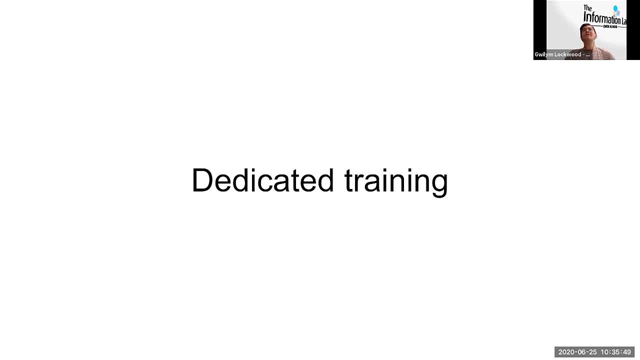 everyone's on about the same level. Like, yeah, it always kind of reminds me of playing sport at school. I absolutely I sucked at all kinds of sport at school and I hated it. And what I always really hated was when it was rugby time in PE. They'd put the kids who were on the rugby team 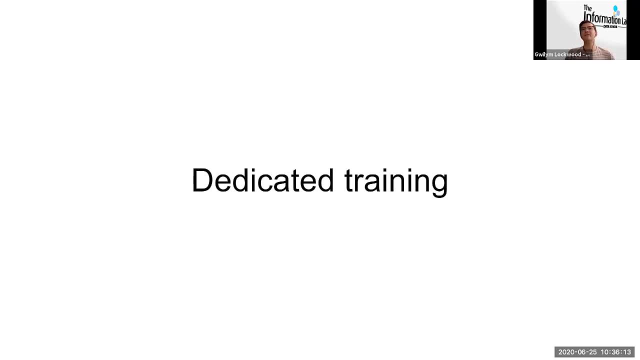 along with kids who are just sort of unfit and skinny, like I was at the time, And it was horrible because you'd just get completely crumpled by these massive units who are trying to train to represent the England under-14s or under-15s or something. That was putting everyone on very different levels in 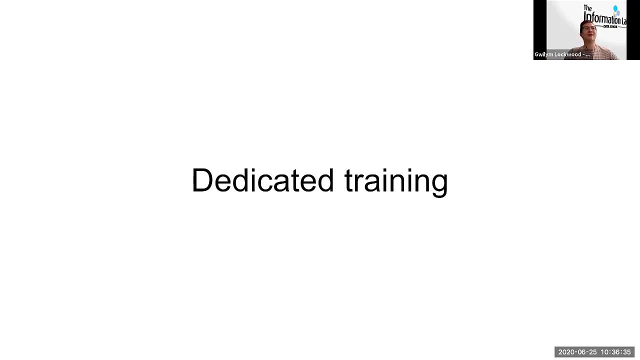 the same situation And the big guys who are training didn't get anything out of it. I didn't get anything out of it, But rugby was so much more fun when they'd, when the teachers were like, okay, we're going to take the good guys off to one side and we'll leave everyone. 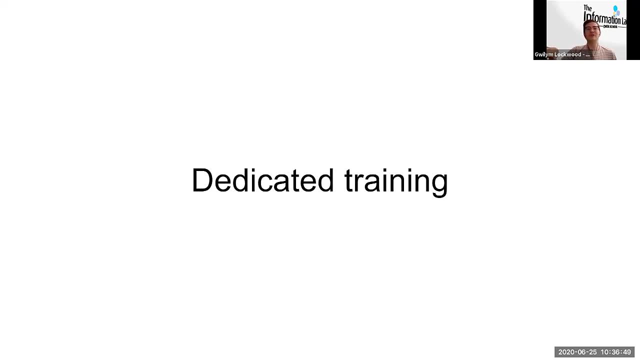 who's kind of crap at rugby in this other group and we'll just do some basics with you. And I was like, oh right, Yeah, we're all at the, we're all on the same level here, And this is actually. 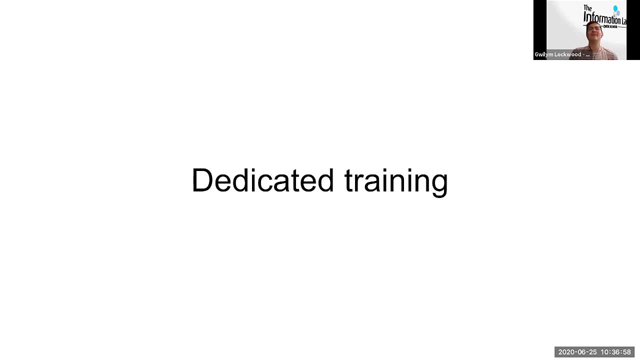 kind of fun now. So that's always what I think of when I'm doing database training sessions. It always takes me back to PE at school, which is kind of odd how deep that runs. Yeah, After dedicated training, there's also the resources option, So this is where you can. 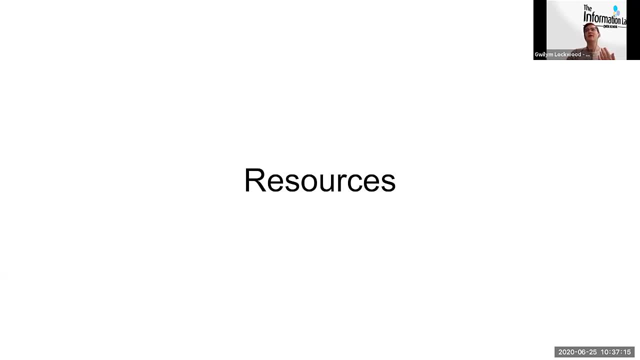 include release notes and diagrams. So when we release a new dashboard, that's particularly complicated, I'll often, as a client, send out an email saying: hey, the latest version of this dashboard is available. You can access it here. Here's some notes about what's new about it, Like: 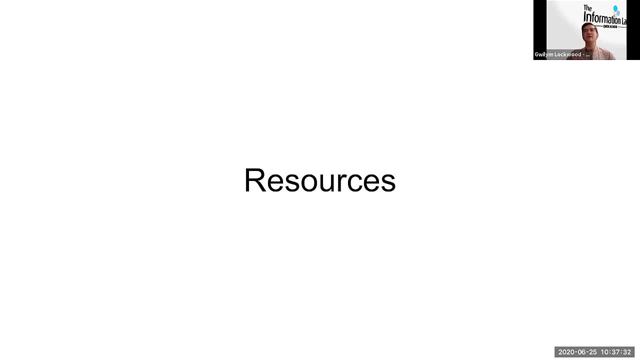 if it's an iteration of an old version, then we'll say: we've included this ability. We've included this new graph that lets you do this. We had feedback from last time that said that people wanted to be able to do this use case And hey, we've managed to get that. 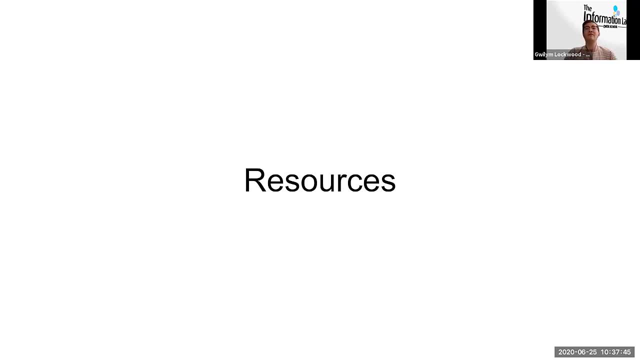 in now So you can see how to do that here. Sometimes we record little videos that show people- either me or the users or someone else- interacting with it to say how they're using it. You also include some release notes, So maybe this is when I'll package up into like a little. 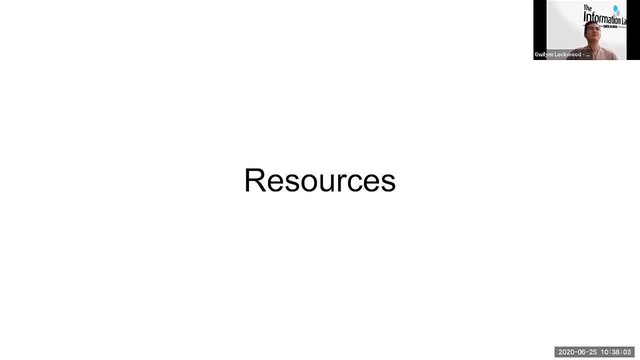 two-page document, the whole z-score thing with the heights and the countries and so on. So, yeah, notes and diagrams in the release notes – that often works as well. Yeah, People that are a little Old-ago, so I don't really get into that stuff. People that: 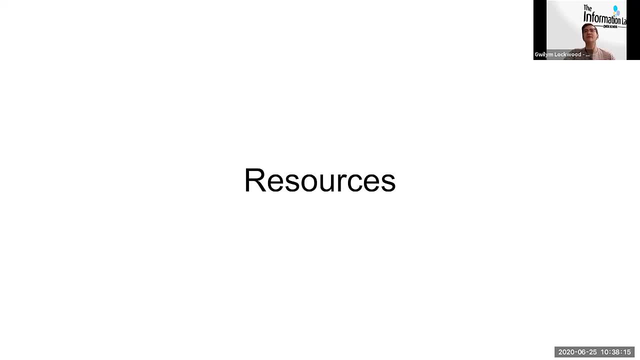 it gives something. it gives people something to come back to in their own time, when they want to, when they want to figure it out. and, yeah, it's funny, it's the human option. um, if you make yourself known as a friendly face who's happy to help, people will just come to you like: um, it's certainly. 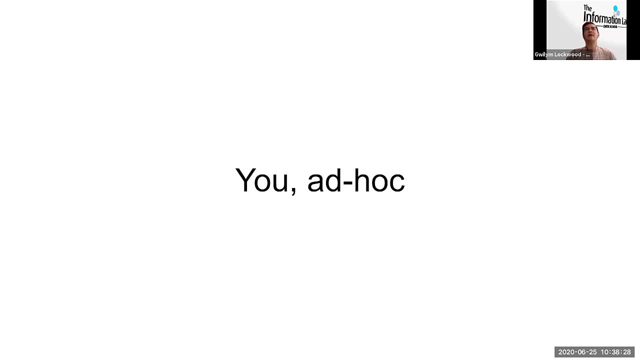 what's what's what works for me, either at the information lab or at clients. uh, once you i find that, um, once you've developed an area of interest and you're just kind of uh happy to help people out, that that becomes a really nice self-fulfilling cycle where if i'm uh, if i've got the reputation- 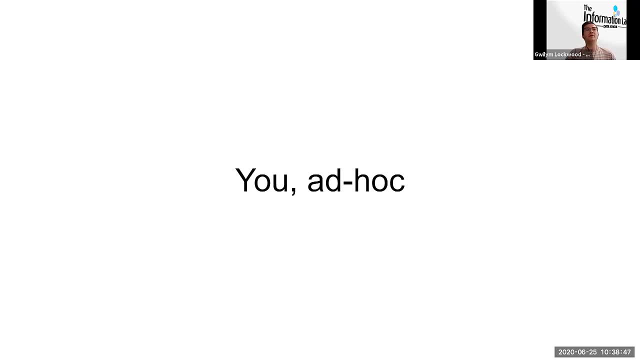 of being, um, like being the stats guy who, uh, is someone who can, can, take the concepts and make it a bit less terrifying. uh, people, people, come, come and ask me about it and i'm always just really happy to help, and then that that, uh, that's um, that that helps people at work or people at 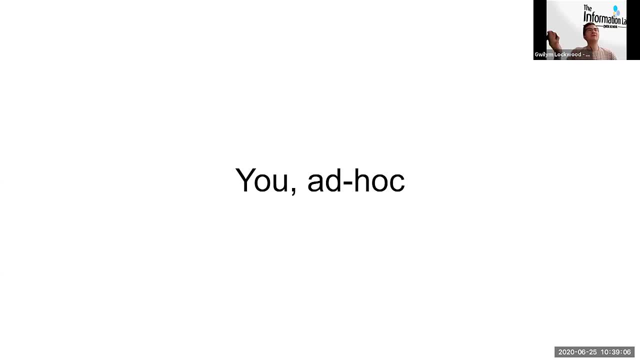 clients, uh, feel more comfortable with what they've done and and it's just, it just works really nicely. uh, i, i love it when people just come to me, uh, and say, hey, um, i'm trying to do this, have you got any thoughts? or hey, i'm trying to do this and i'm i'm stuck at this point. have? 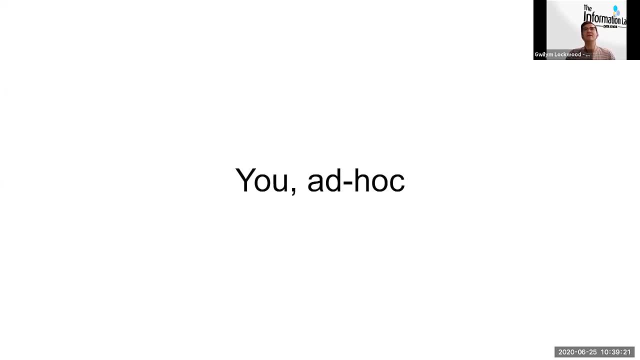 you seen that before and and it's great and that that just helps everyone because it helps me get better at um- more stats training if i'm going to train that thing in the future- and it helps that person gets better at the thing they're trying to do there. so that's the third option: the human. 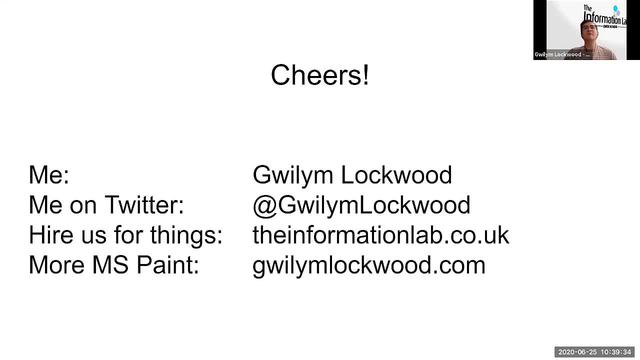 option, and that's pretty much it for today. so i just want to say thanks, thanks for turning up. i appreciate that it's, um, uh, still really nice and sunny outside. it's definitely where i'd like to be, uh it. i think we're all getting. we're all starting to get maybe zoom fatigue as well, uh. 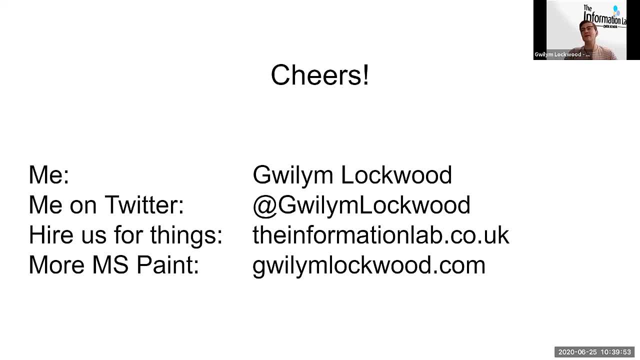 so it's great that there's so many different things going on- there's so many different webinars and online conferences and stuff- but it also means that there's a there's a lot to choose from, so i'm really glad you chose to first to tune into this one today. yeah, so again, i'm william. 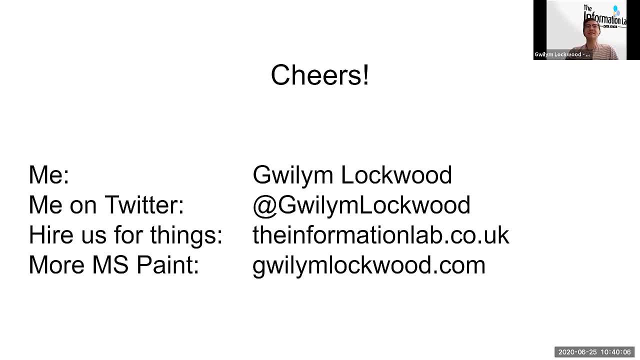 lockwood. if you want to find me on twitter, it's just my name. i'm incredibly easy to find. uh, if you want to hire us to do things, we're at theinformationlabcouk, and if you want to see more microsoft paint diagrams, i've got a lot of those for various different things. just on my 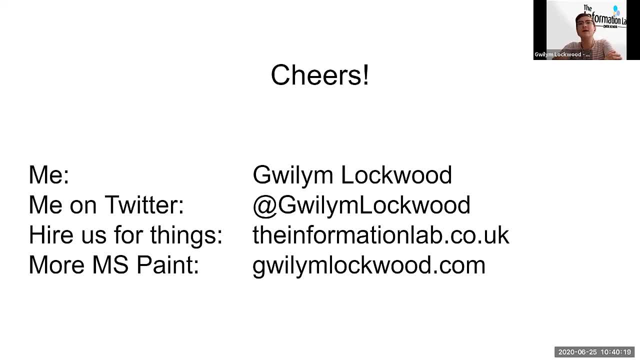 website, which is again just williamlockwoodcom. all right, that that's it for me, i think. i think we're going to do some questions now. uh, sophie, over to you. hey girl, i'm just making sure i've unmuted myself there. yep, um, we don't have any questions in the uh. 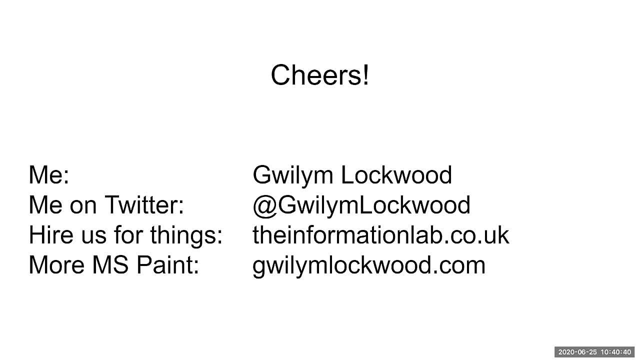 zoom chat. yet, um, we've just, uh, had tim beard um say he he lives in germany and germany is also pretty, pretty direct. um, i have some questions for you. so if you have any questions, um, please type them into the chat for willem to answer. but just as we give everyone a moment or two to 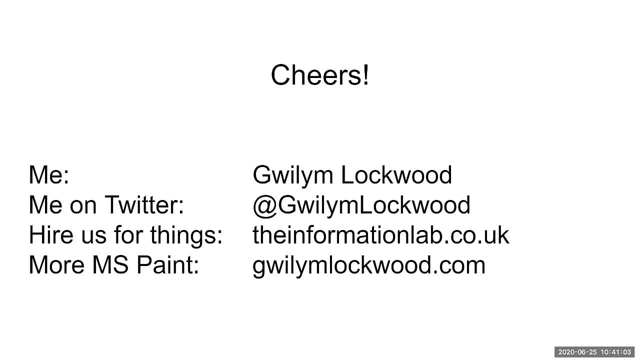 warm their fingers up and type into the chat box: willem, yeah, how, how long does it actually? i love microsoft paint pictures and i think they they also add an element of humor, but they're also not very precise, which is which is good. it makes it feel um, makes the concepts you're conveying feel. 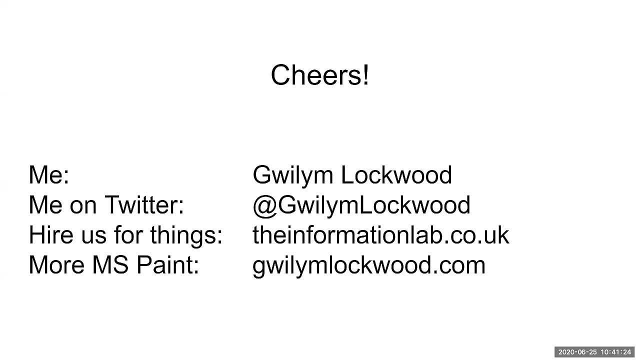 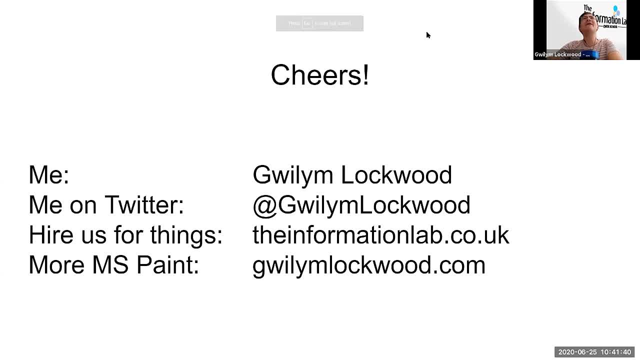 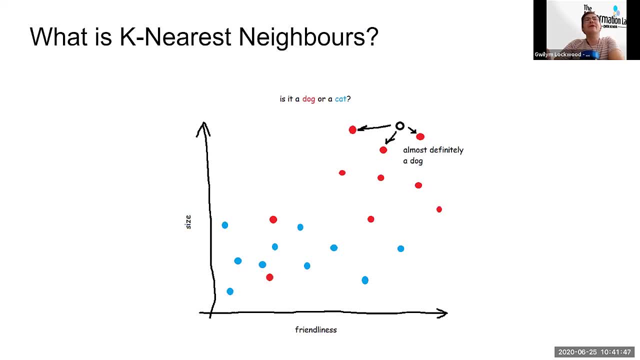 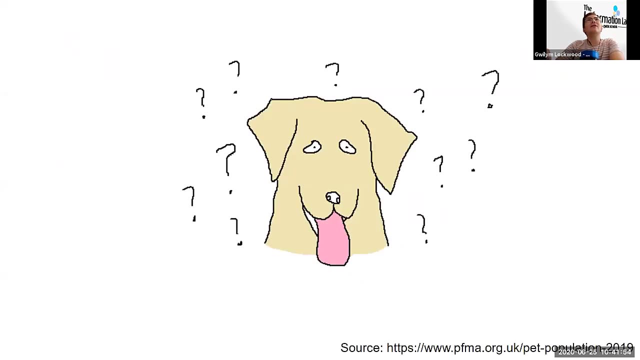 that's why it looks so uh, hurried and unprofessional. i, i will admit, uh, let me scroll back to some um like these, took no time at all. um, the, the the. the time that this took was making sure that i understood the concepts before drawing them. uh, the the dog took a little. 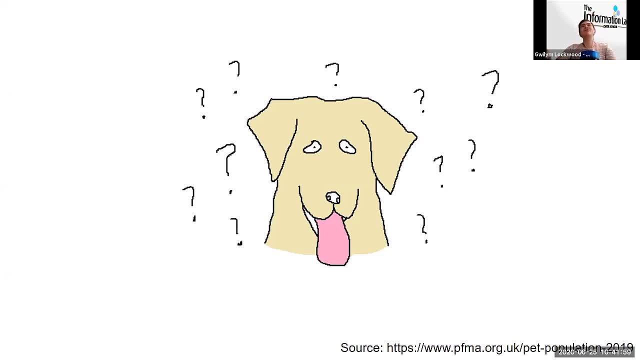 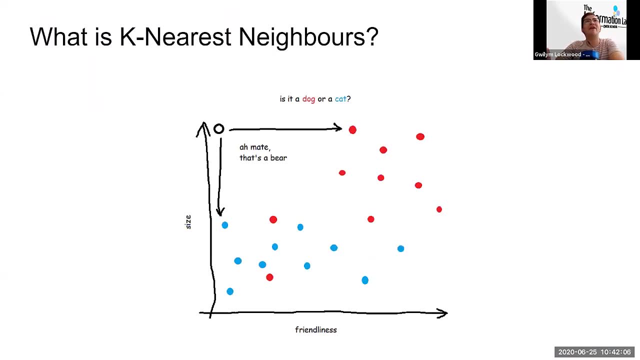 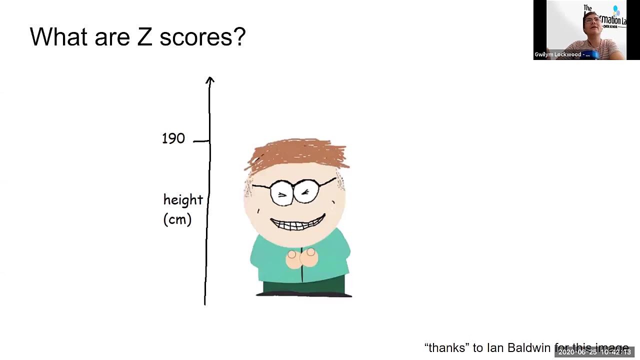 while longer to draw. i want to say that the dog took me about 15, 20 minutes, because i've never tried to draw a dog before. but, um, but, yeah, the uh, the anything like this is five minutes. um, yeah, uh, this one, uh, okay, the one, the self-portrait in my face, that was, uh, that was. 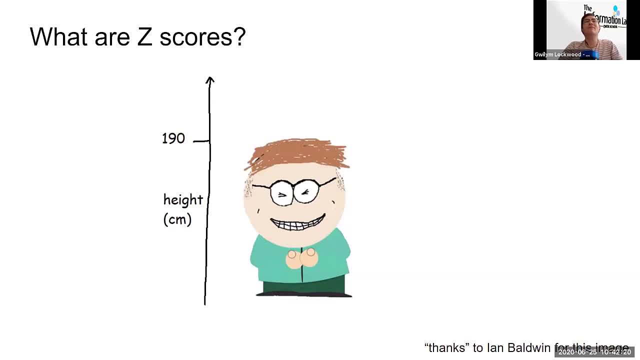 something i spent a little while on, because it was, it was for a, it was for a project for a friend and i just, but then i can just copy and paste it everywhere else. and then the um, uh, it was originally just in black and white, and then, um, ian, at the information lab, uh, superimposed it on top. 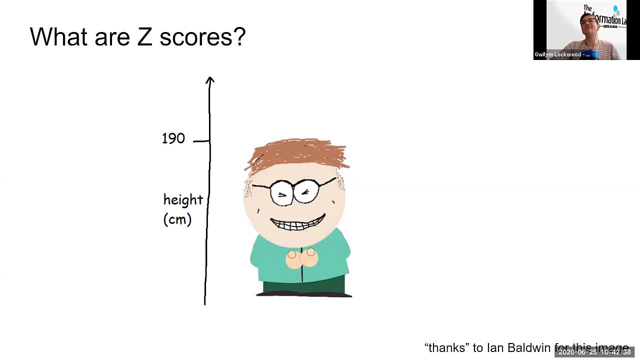 of the um, like the butters from south park on top of butter's body, and i was like, oh yes, you're not wrong, i've got to use that now. so this one took no time because i just copy and paste it. so on average we, so they don't take as long as they they look they might. 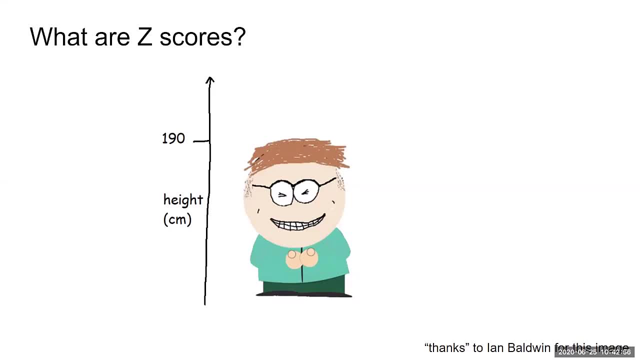 look like they could. i know i'm not very good with drawing with my, my mouse and microsoft paint. um, yeah, five, ten minutes tops, uh. uh, not a question per se, but um had a. i wanted somebody say: um, how do they subscribe to your blog? um, they've said they found it, but uh, if people 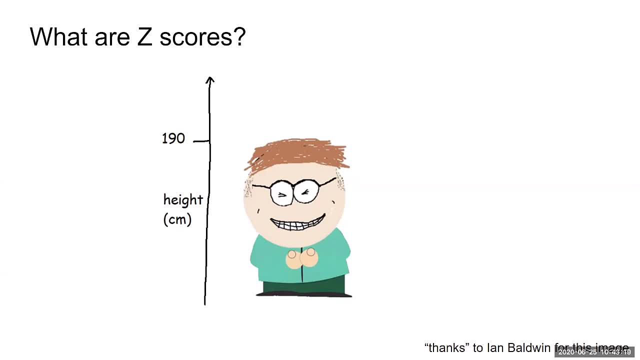 are interested in subscribing or hearing, um, more from you is the best way to subscribe to your blog or an rss feed, or to follow you on social. i put the you on twitter. yeah, i'd say linkedin up there as well. twitter's probably the best bet because if i, if i post, 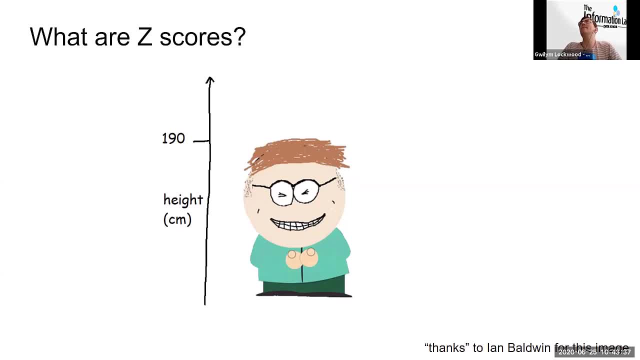 something on my blog. i'll probably end up just tweeting about it, but, um yeah, i'll be honest. my, uh, the my knowledge of web development or just web infrastructure in general is relatively minimal. so i have, uh like, i just set this blog up with wordpress because it made it easier for 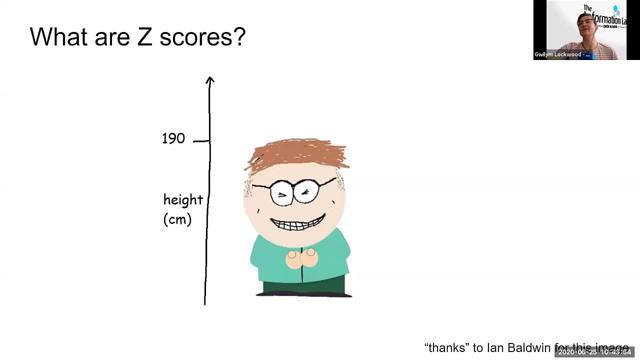 me and i have no idea how to do a website properly. so, uh, i i guess it's possible to subscribe to the blog, and yeah, all those things could, and yeah, help me out some more, but hanging out at once or, you know, have other questions. however, have you got real fun? you do. 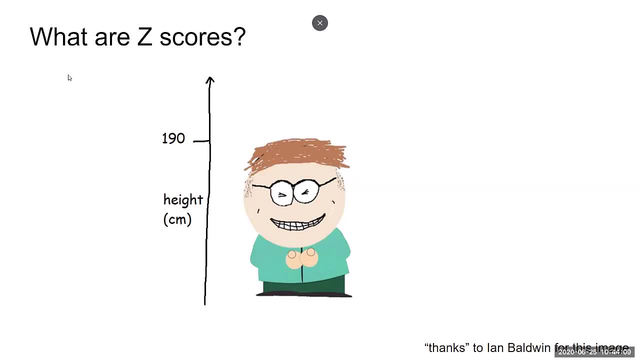 use our rss feed. um, we're upgrading rss, but we use the voting rss, but i've never used rss feeds before, so honestly i don't know. perfect, okay, and um, last question, just because we're coming up in time: um, how, um, what reactions have you got to from, from clients, if you showed us some, some of? 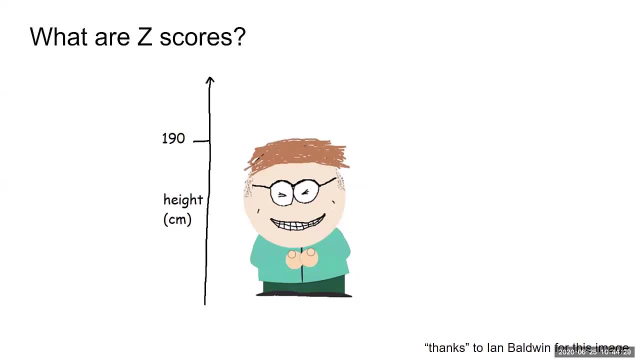 your microsoft paint drawings and then real life and the charts. have you found it's really helped them understand the concepts or are they generally yeah, um, yeah. i've only had negative reactions to microsoft paint diagrams once or twice before in in like very, very serious institutions who are like above this kind of thing. um, the the majority. 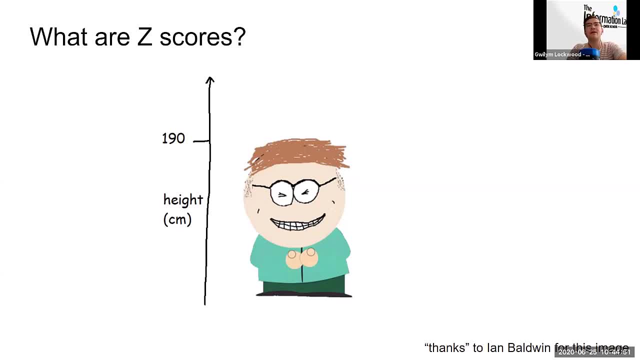 of the time, people are like: uh, oh, yeah, i guess this is just the exact same thing as scribbling on a whiteboard, but in in a way that you can stick in an email later on. it's uh, yeah. most most people are just like: all right, yeah, cool, this is. uh, this is just like drawing something. 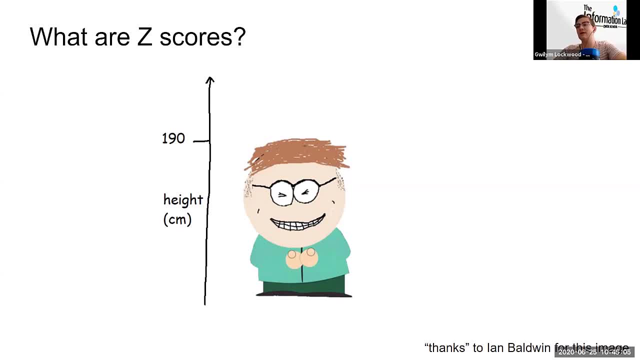 on a whiteboard and and uh and playing around with ideas and and i i think that a lot, of, a lot, a lot of people love it when you can, uh, scribble stuff on a whiteboard together and and explain concepts like that. so, yeah, most people just take it like that and enjoy it- perfect. so 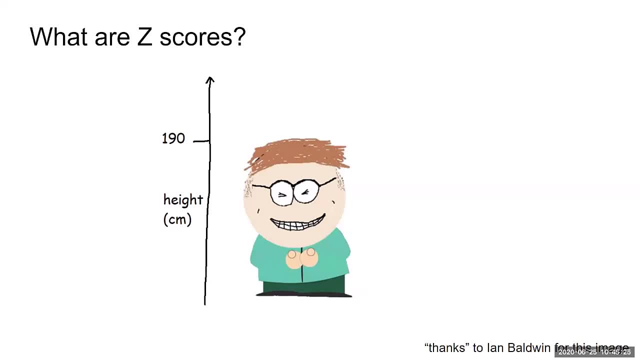 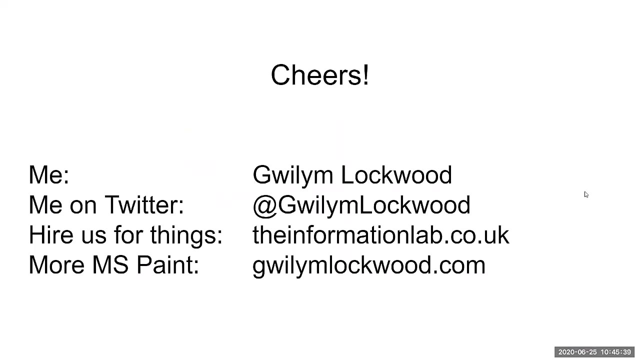 um, that's us on time. um, if you do have any other questions, please reach out to guillem um on his email or on social um. he showed the. uh, guillem, actually can you go forward a few slides to your contact details again? um, so you can reach guillem if you have any questions on any of these uh. 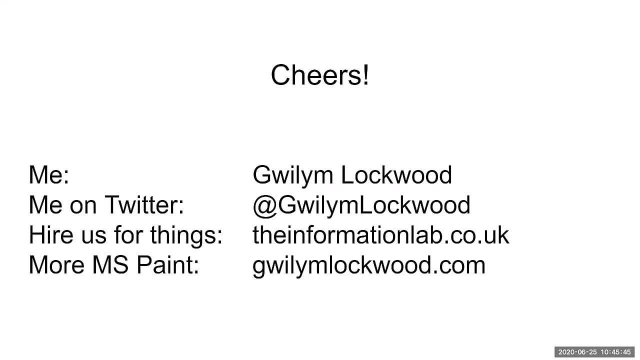 forums, twitter, um his uh through the information lab, um more on his blog or i've also put his linkedin link further up in the chat. this um session has been recorded so i will post the video in the next day or so and put the link in meetup. so, if you have, if you want to re-watch it, 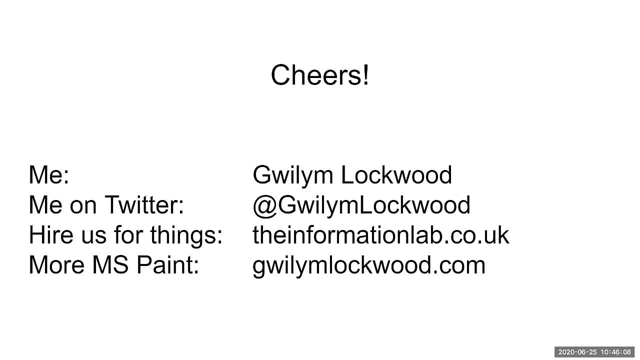 um, you'll be able to. and lastly, if you would like to learn more about how to make concepts, um, about anything more approachable, or any of these similar um themes that guillem is, uh, quite expert on, please do let us know in the comments on meetup or reach out to guillem directly, because 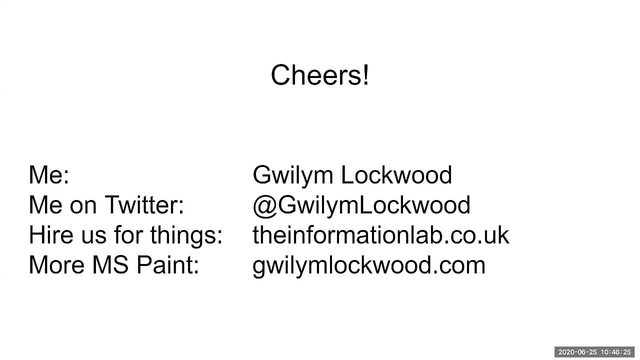 this is a explain uh. simplifying and explaining concepts is something we all need to do, a lot as we, as the audience for our work, gets larger, and this is something we'd like to be able to help you to do, so we could have some future events that are similar. so, before we stop, um, there's uh. 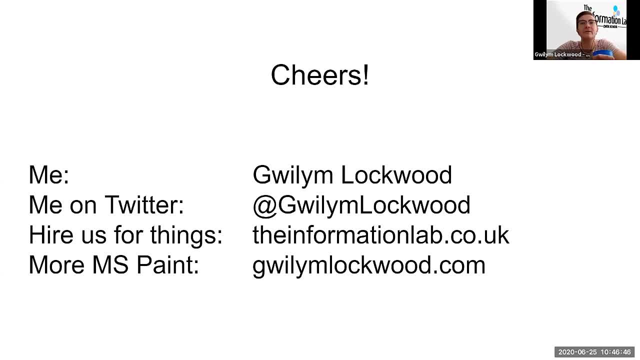 there's one question that's come up in the chat that i can answer quickly from from tara, saying: do you think it's important to have a math stats background to work in database? a lot of job roles ask for math to highlight level uh, any tips or suggestions for this? can i answer that one quickly? 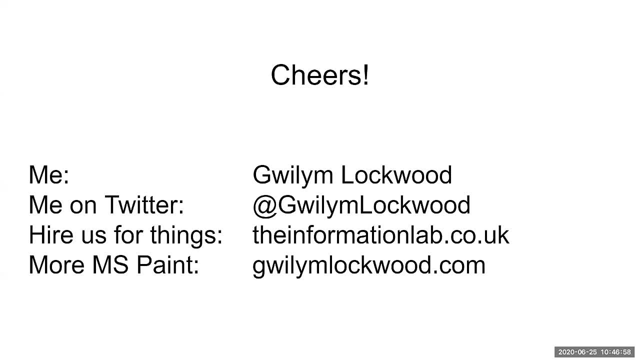 for sure, for sure. yes, i don't. i don't think it's absolutely necessary to have, uh, a math stats background to a high level, but i think it's important to be open to learning it. so it's um, like: there's, there's a lot, of, a lot of things in database don't necessarily require. 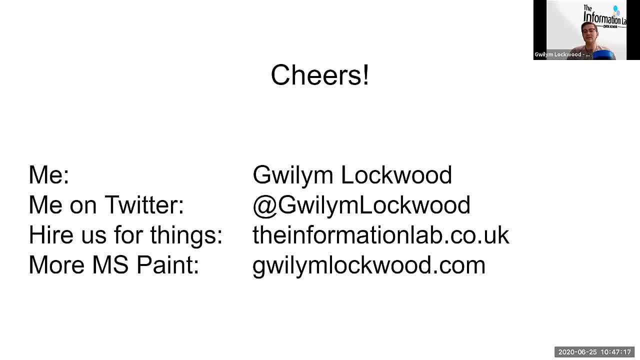 maths understanding like you can uh. you can create a bar chart, you can create a scatterplot, you can create all sorts of interesting dashboards without under uh, without uh, you know any kind of advanced qualifications in maths, but at the same time, i think that um you. 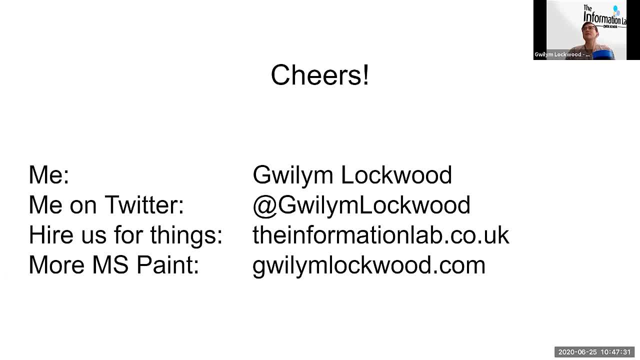 there are a lot of decisions that get made, uh like maths decisions or stats decisions that that get made that you should have an understanding of. like um, i want one of the simplest is just the uh, just knowing whether whether to use a mean or a median like um. i remember for a client i was 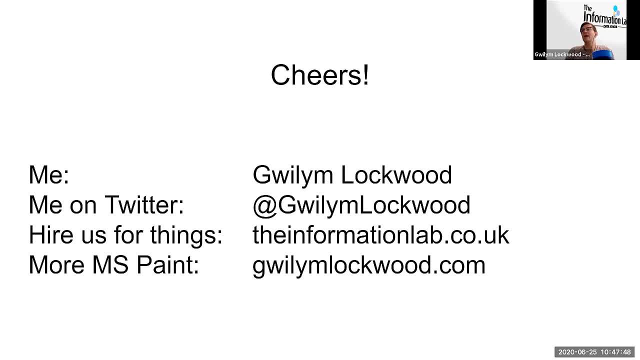 doing some. uh, i was doing some gender pay gap reporting at one point and, um, there was, uh, there was this one particular section where i had to report: whether does this organization have a gender pay gap? and the. the interesting thing is that if i use the, if i use the mean to to report. 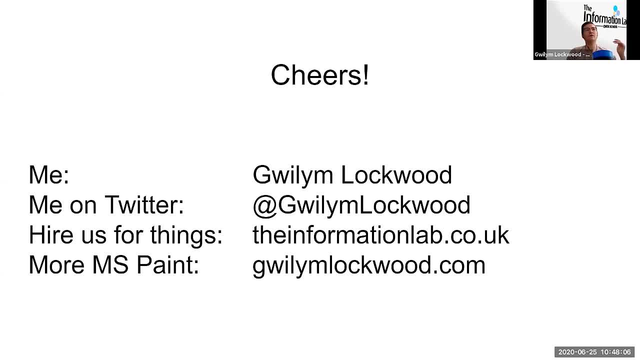 it then there was a gender pay gap in favor of men and, if i use the median, there was a gender pay gap in favor of women. so, um, it's like the uh the. i think the main thing that you need to do in situations like that is is knowing that, um, not just assuming that every kind of out of the box. 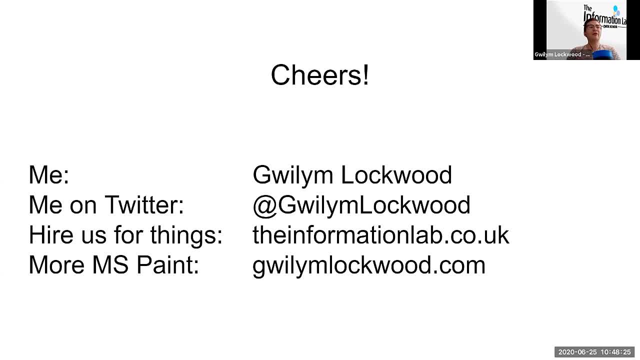 option is, um, uh, automatically right, but, but knowing enough about uh, having the instinct to maybe not instantly trust everything that database software is telling you instantly, and having enough understanding of maths and stats, think, okay, hang on, let's explore different approaches to make sure that i don't just interpret this uh at face value. so, uh, i guess. 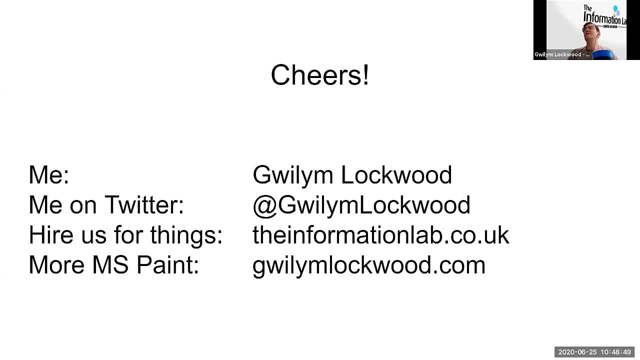 what i'm saying is that the knowing maths and stats to a high level isn't necessarily essential, but, uh, you should be able to compensate for that. or actually, even if you do have maths and stats to a high level, you should always have the kind of doubt in the back of your head that goes hang on. 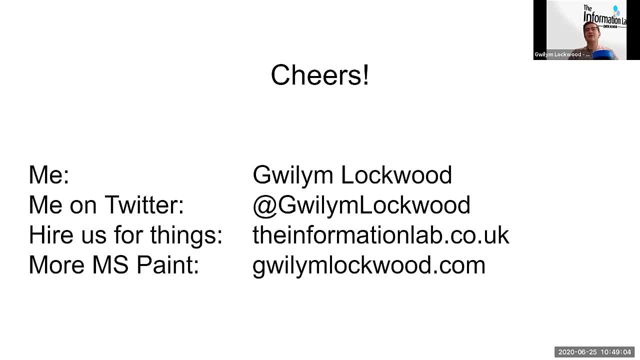 a second. let's not instantly uh trust this and take it as face value. let's explore different, um different options to uh try and to try and get a more nuanced take on things before just making any kind of absolute declaration of anything. so, uh, yeah, to summarize, i'd say, uh, you don't. 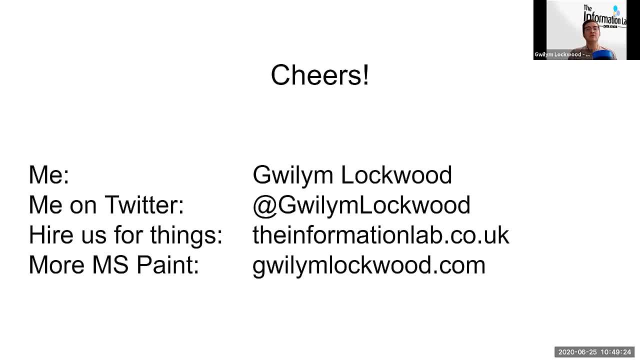 necessarily need to be able to make any kind of absolute declaration of anything. you don't need to be able to make any kind of absolute declaration, you just need the high maths stats background. but you do need to be open to it. you do need to be open to learning, uh, more stuff, because it will. 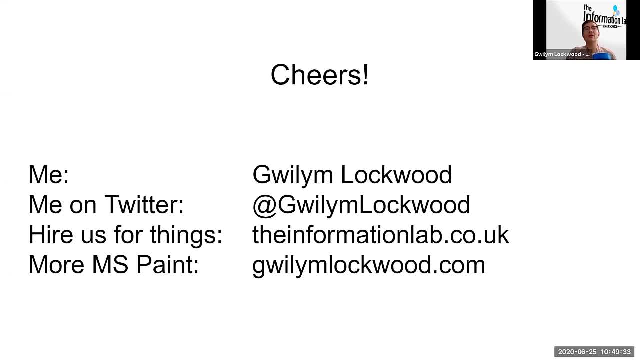 come up and there will definitely be situations where, uh, a solid mathematical understanding will be really important for some analysis that you're trying to do. so, yeah, and, and a lot of this you can learn on the job, but it is, uh, it is something that will come up.